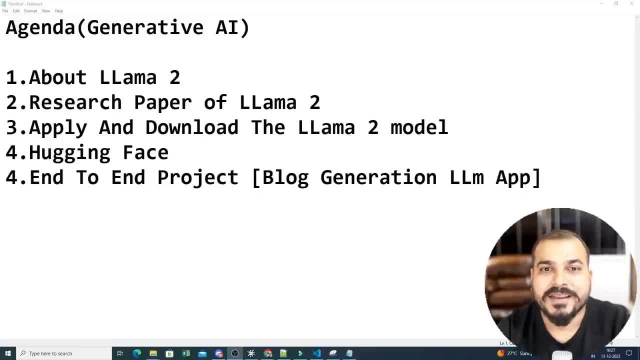 Hello all my name is Krish Nayak and welcome to my YouTube channel. So, guys, yet another amazing video on generative AI, where I will be specifically discussing about Lama 2.. Lama 2 is an open source model. Again. it has been created by Facebook or Meta And you can use this specific model even for commercial purpose, So this is quite amazing. This is an open source LLM model altogether. I will try to show you how we can use this. 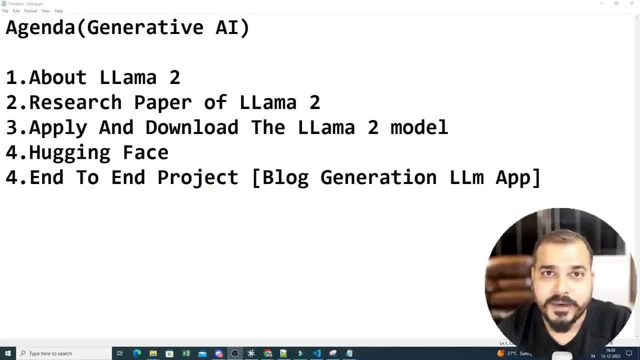 Create an end-to-end project, also in this specific video. So there are many things that are going to happen and probably whatever topics that I teach going forward that is related to generative AI. I will definitely follow this kind of approach so that you also get a brief idea about all these kind of models. So what is the agenda of this particular video? The agenda is that we will get to know about Lama 2.. Then we will go ahead and see the research paper where I will be talking about the key points about the Lama 2 model. 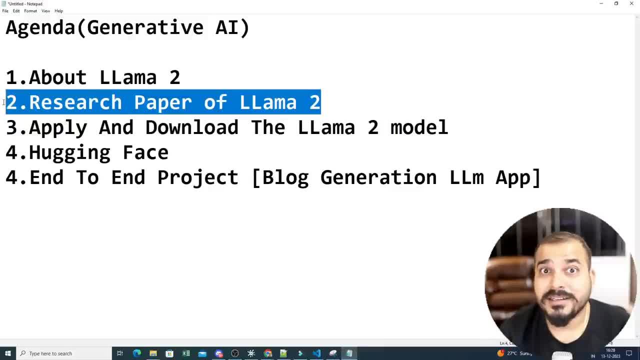 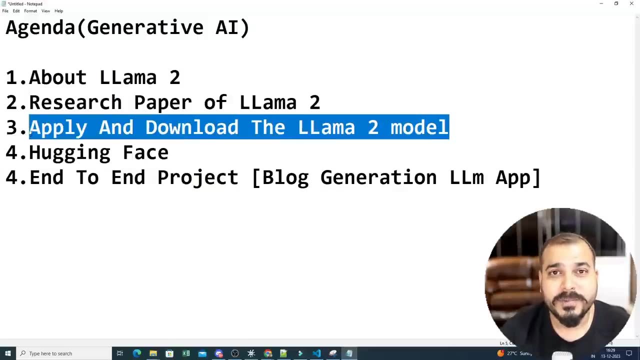 Again, since this is an open source and soon Lama 3 is also going to come up. So that is the reason I'm going to create this particular video. I really want to be in sync with all the open source LLM models that are coming up. Right, Then we'll go and apply and download the Lama 2 model, So we'll be seeing like how we can actually use this particular model in our project also. So for that purpose, I will be downloading this model. You have to also apply this in the Meta website itself And there is also one way how we can also use it directly from the LLM website. 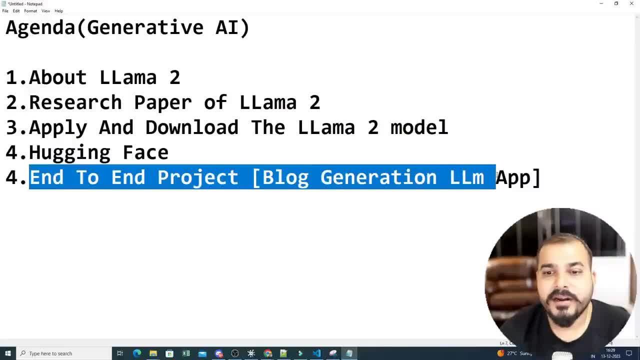 hugging face. so i will also show you that, and after that we will try to create an end-to-end llm project and this will be a blog generation llm app. all these topics i will be covering it. i know it will be a little longer video, but every week one kind of this kind of video is necessary. 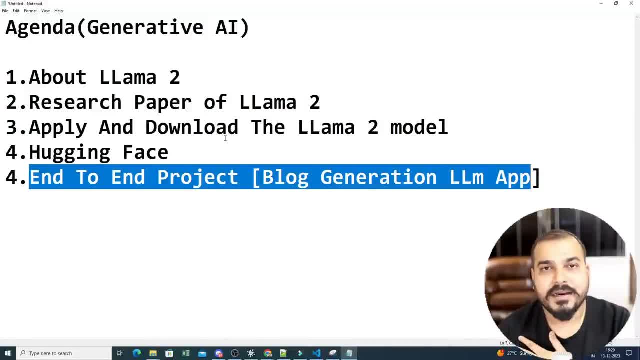 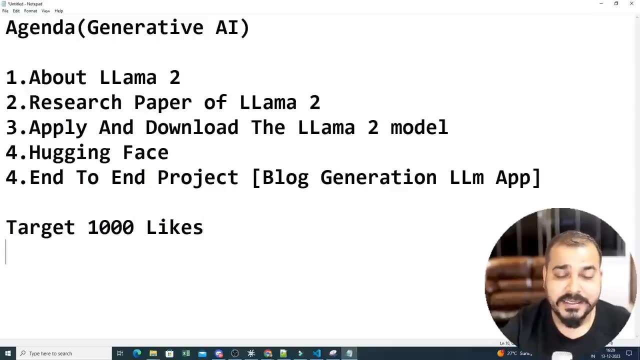 for you all and since 2024, i have the target. i really need to teach you generative ai in a way that you can understand it and use it in your industries also. so i will keep a target. so every video, i'll keep a target like this. target for this particular video is thousand lakh likes. 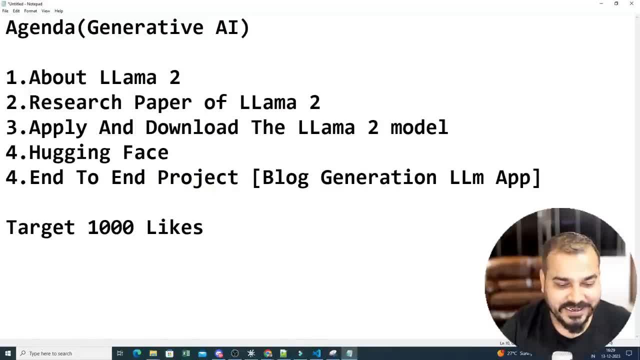 not thousand lakhs, but thousand likes and comments. please make sure that you write some comments and i'll keep the target 200, okay, so this will actually motivate me. this will probably help this particular video to reach to many people, through which they can actually use this, and 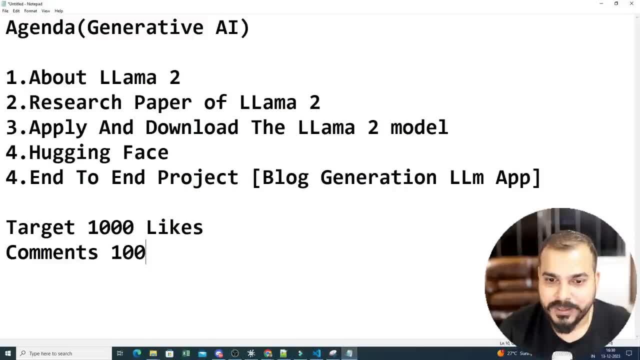 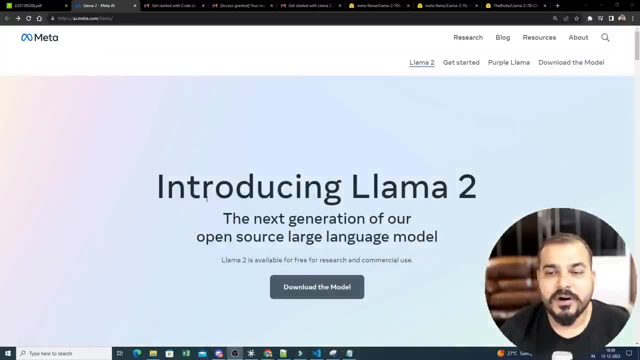 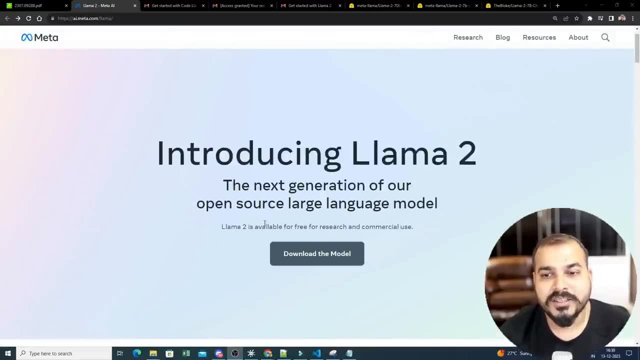 entirely. this is completely for free, which will also be beneficial for you and i have. my aim is to basically democratize the you entire ai education. okay, so let's go ahead, and let's first of all start with the first one, that is, introducing llama 2. what exactly is llama 2? llama 2 is an- again open source, a large language. 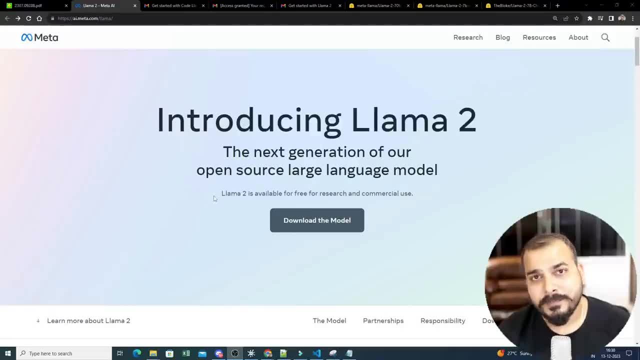 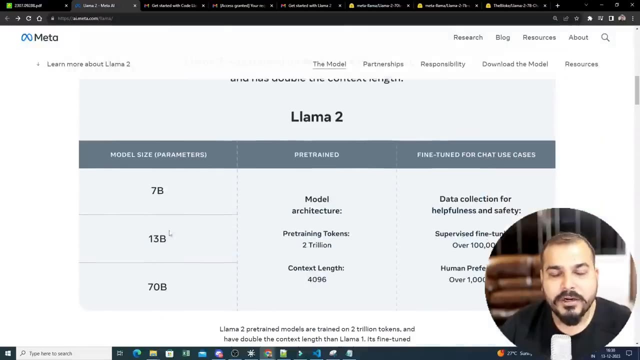 model it can be, it is used and it is uh available for free for research and commercial purpose. you can actually use this in your companies, in a startup, wherever you want to use it. okay, now let's go ahead and read more about it. so, inside this model, uh, it has till now, llama 2 has released. 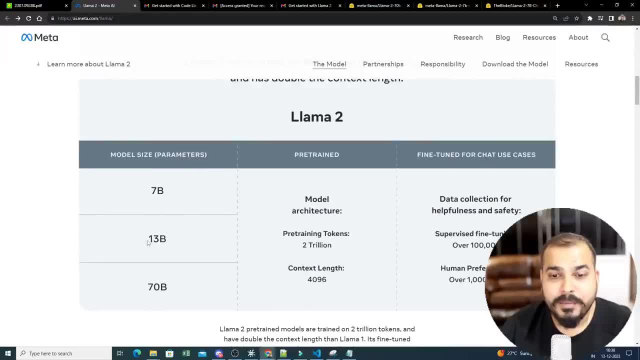 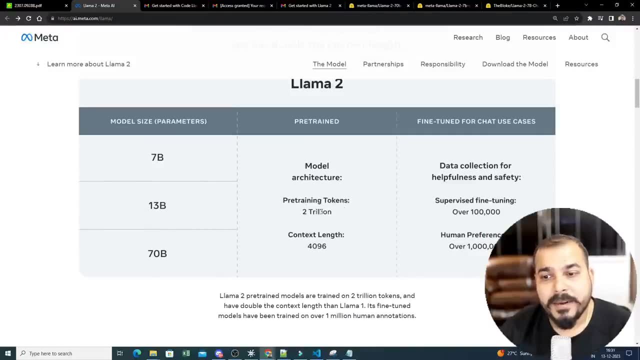 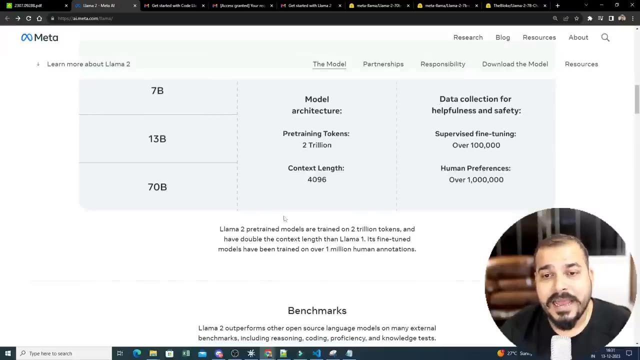 three different model size uh. one is with 7 billion parameters, the other one is 13 billion parameters and the best one is somewhere around 70 billion uh parameters. uh pre-training tokens is taken somewhere around 2 trillion. context length is 4096 uh. again, when i say that, if i probably compare, 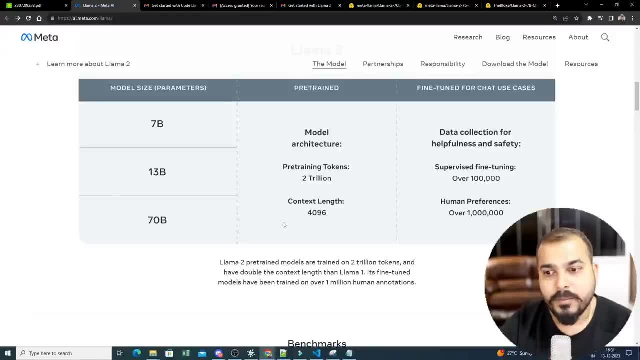 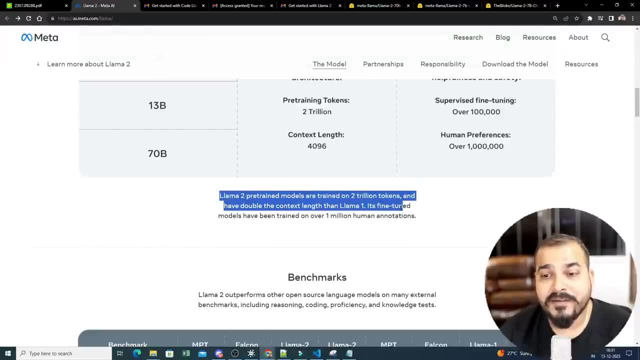 most of the open source models. i think llama 2 is probably very good. we'll be seeing all those metrics also. so here you can see lama 2. pre-trained models are trained on two trillion tokens and have double the context length than llama will for one. its fine-tuned models have been trained on over 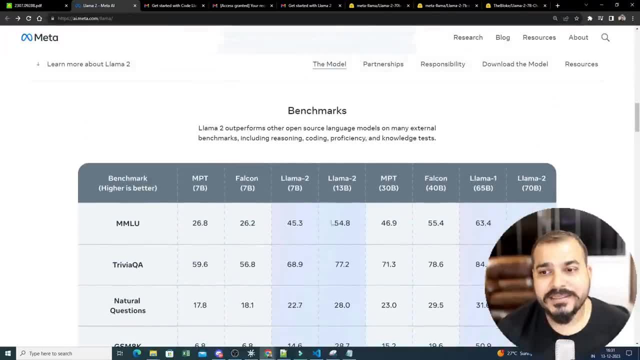 1 million human annotation. okay, and now let's go ahead and see the benchmark. and this is with respect to the benchmarking with all the open source models. so it is not comparing with chat, gpt- sorry- gpt 3.5, gpt 4.0 or palm 2- okay, so all the open source models. uh, here you can probably 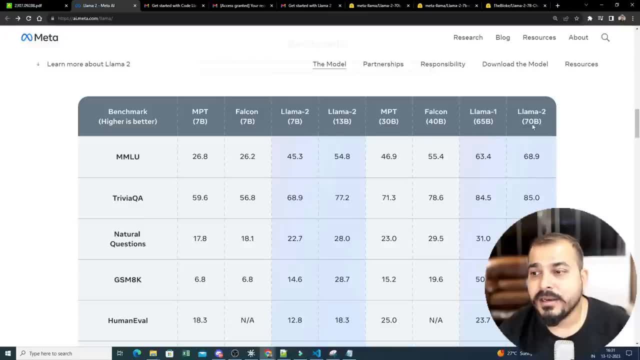 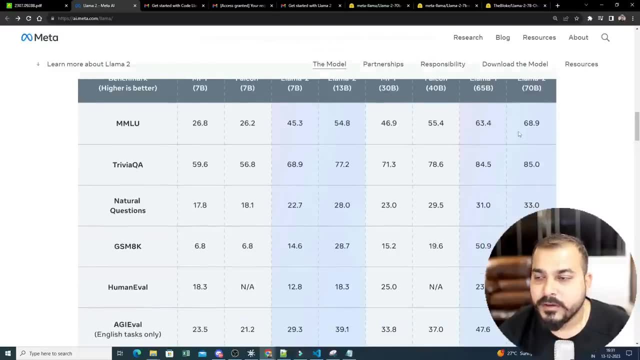 see, this is the three version: 7 billion, 13 billion, 65 billion, 70 billion, right all llama 2, right llama 1 was 65 billion, one, uh, one model it had over there. so if you see, lama 2 with respect to all the metrics is very good. mmlu, that is, with respect to human level understanding, q and a. 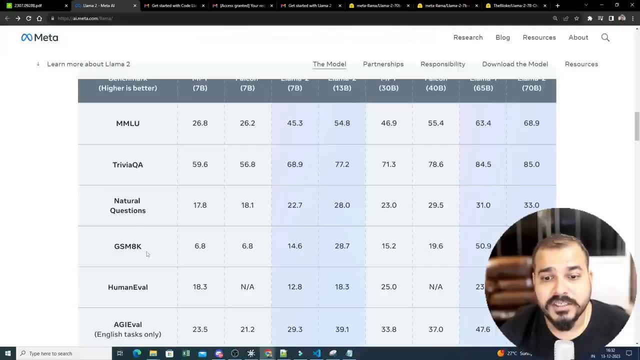 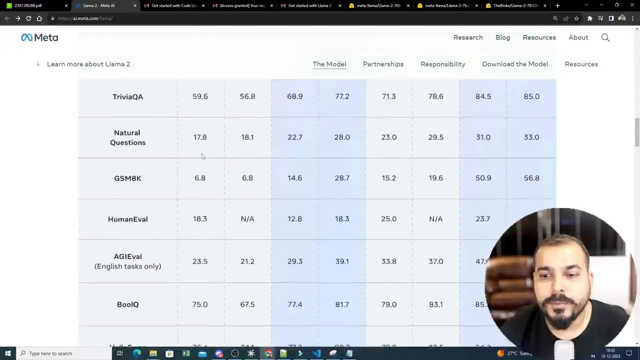 all, all the performance metrics is superb. natural language processing, gsm 8k human eval. in human eval it is probably having a less when compared to the other other open source models. so here you can see in human, uh, human valve, human eval. human eval basically means with respect to 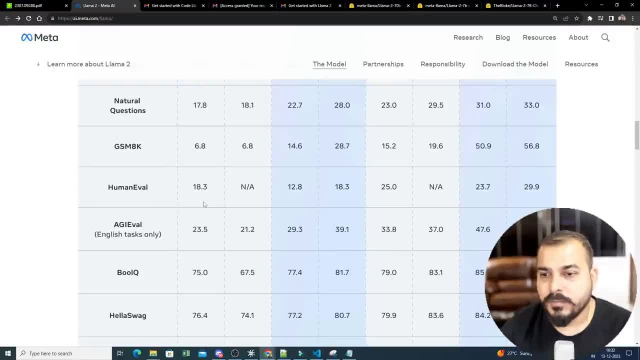 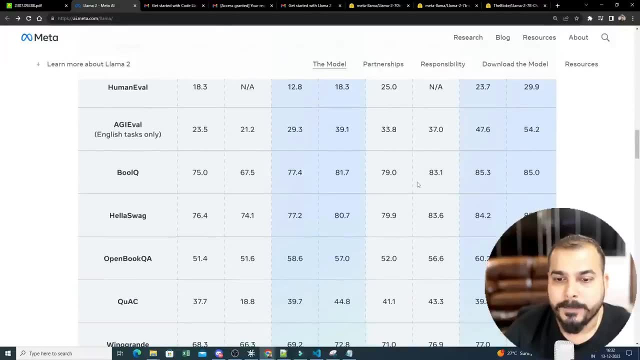 writing code, code generation. there it has a lot of problems. so here you can see 12.8, 18.3. it is less. it is less when compared to all the other open source models over here and there are also some other parameters you can probably see over here with respect to different. 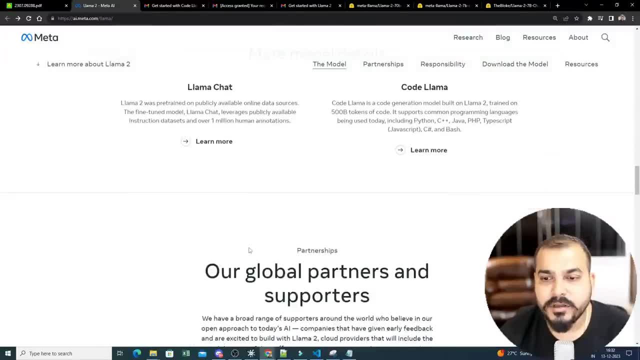 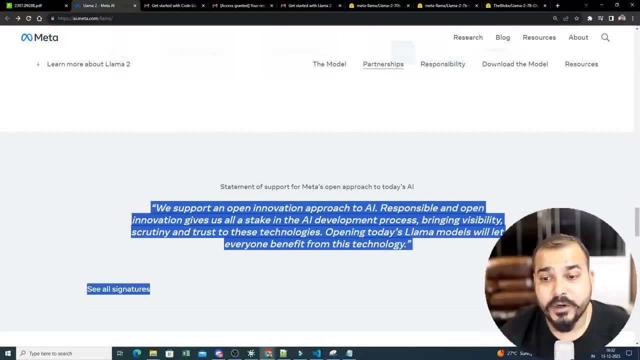 different tasks. you can see the performance metrics. okay, so this was more about the model. now let's go ahead and probably- and this is one very important statement that they have come up with- we support an open innovation approach to ai. responsible and open innovation give us all a. 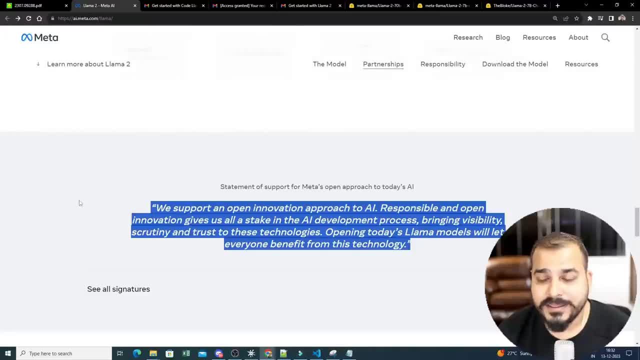 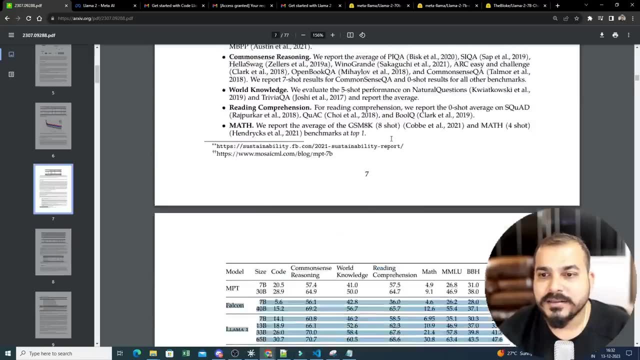 stake in the ai development process. so, uh, yes, facebook is again doing a very good work, and then, soon, they are also going to come up with the lama 3 model. now let's go ahead and see the research paper. so here is the research paper, the entire research paper. now see, uh, what you should really focus on. 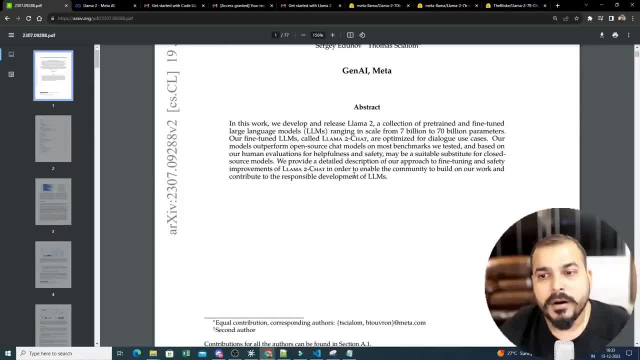 a research paper. you know, in research paper they'll be talking about how they have actually trained the model, what kind of data points they have they actually taken in order to train the model, and all right. so over here you can see that, um, in this work we developed and released. 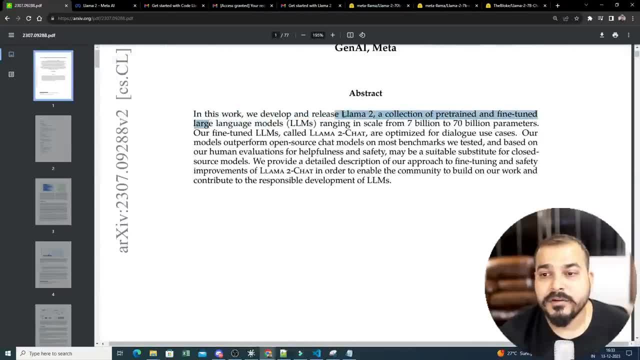 lama 2, a collection of pre-trained and fine-tuned launch language models ranging in scale from 7 billion to 70 billion parameters. so if we talk about parameters, it is somewhere around 7 billion to 70 billion. our fine-tuned llms, called lama to chat, are optimized for dialogue use cases just 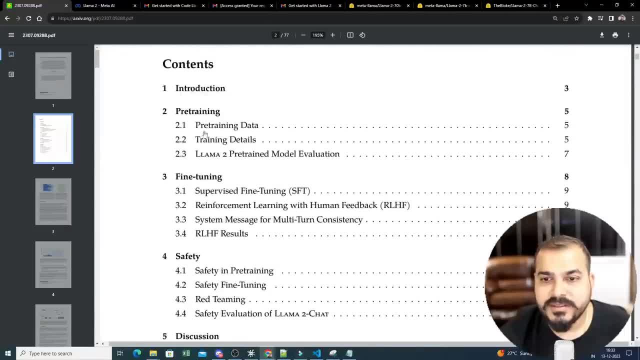 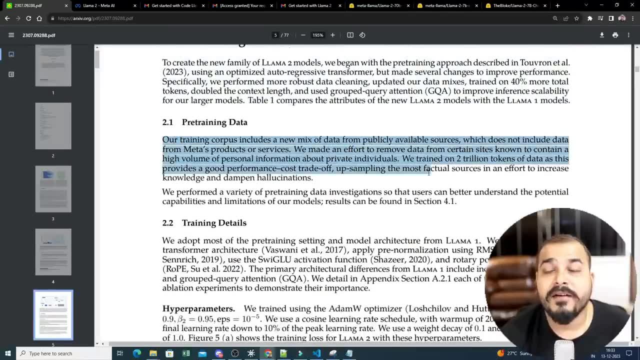 like a chat bot and all right, uh, more information. you can probably see over here what is the pre training data see? so they have told that our pre-training data includes a new mix of data from publicly available sources, which does not include data from meta products or services. we've 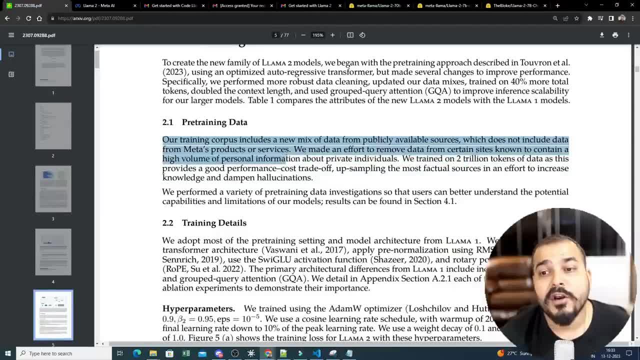 made an effort to remove data from certain sites known to contain a high volume of personal information about private individuals. now, this is where ethics comes into picture. they really want to use this ai in a responsible way, right? so we trained on two trillion tokens, uh, and obviously. 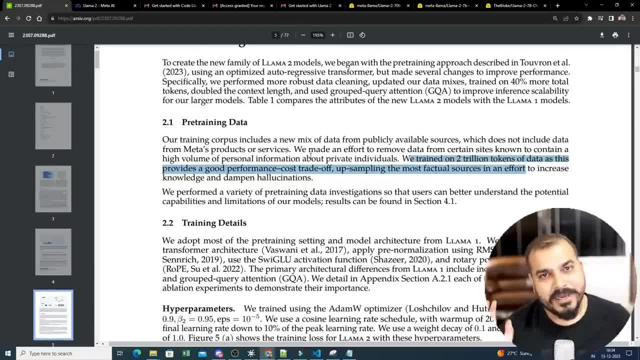 for all these things you have to use nvidia gpu. okay, i know, guys, it is boring to read the research paper, but it is good to have all this specific knowledge, so please keep your energy up. watch this video till the end. then only you'll be able to understand things. 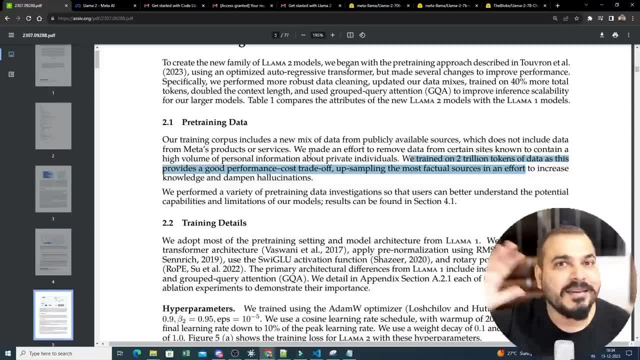 right, not only here, because later on you'll be having other models like mistral. i'll probably create a video on mistral also in the upcoming video right. so everywhere with an end-to-end project, everything. i will take this format. let me know whether you are liking this format or not. 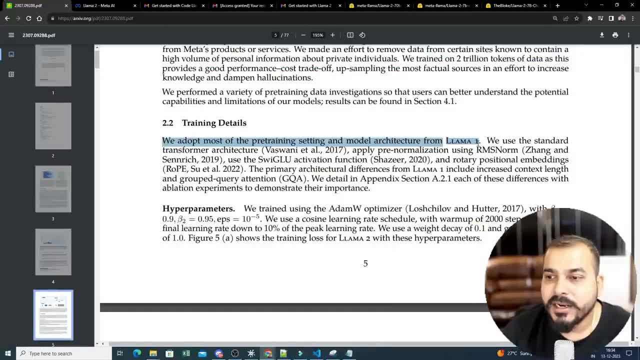 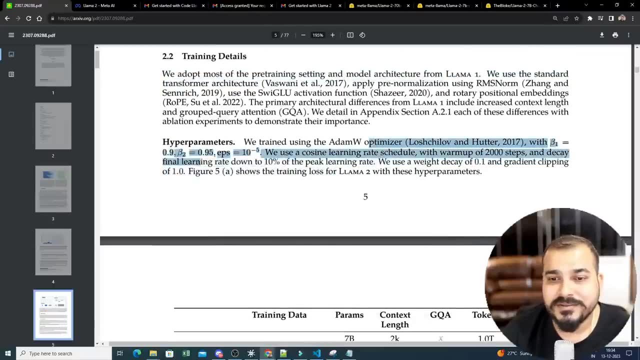 so training data, we adopt most of the pre-training settings and model architecture from lama one. we use the standard transformer architecture. now you can understand how important transformer is. right, most of the open source models are based on transformer architectures itself. right, we trained using adam w optimizer. okay, with so and so parameters, we use cosine learning rate. 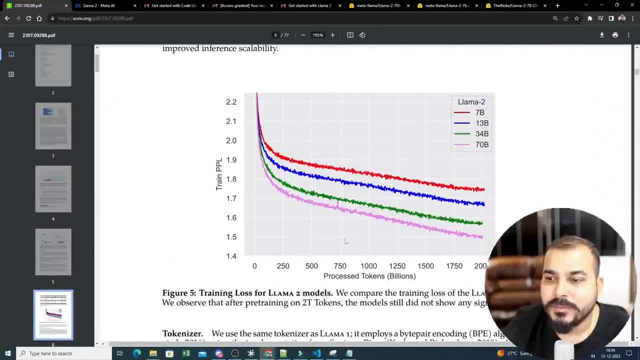 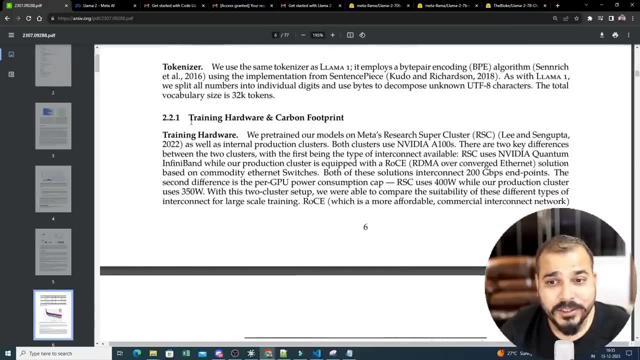 schedule with so and so, and here you could probably see with respect to the performance, like how well it was training ppl process tokens, how many tokens was actually done with respect to all the different varieties of llama model. now this is basically the training loss. you can probably see training loss for llama 2. okay, this is also important training hardware and 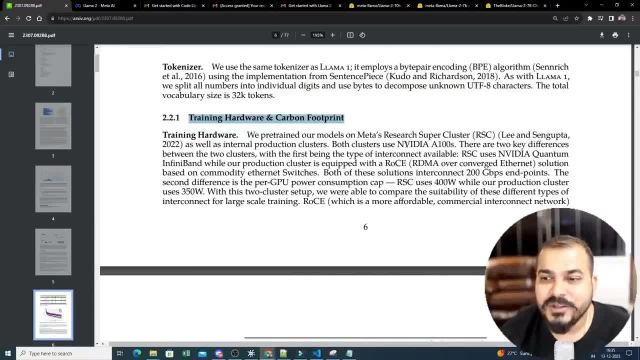 carbon footprint. it is basically saying that how much it is using. they use nvidia, them and data over dials, right, so in a cluster, exactly 800. i've seen this gpu. it's quite amazing. it's very huge, okay, and it is very fast also, but again, with such a huge amount of data, it is also 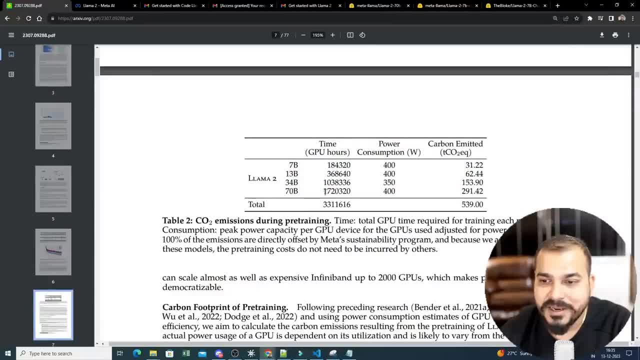 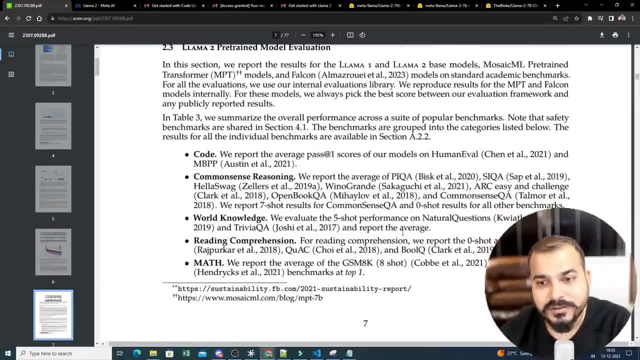 going to take time, right? so all these things are there. you can also see time, how much time it has basically taken, how many hours, 70 billion, this many number of hours, power consumption, this, this, all information is there, right? this is good to have, right? all all you should know, like we're. 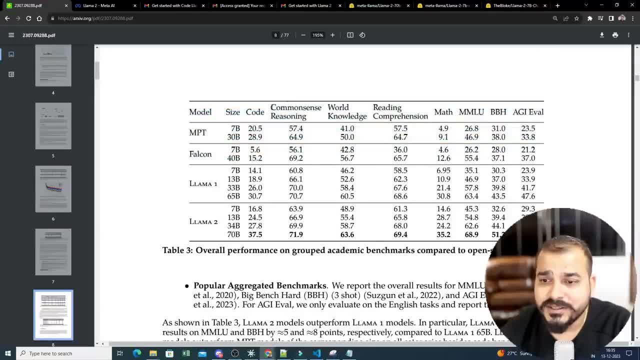 just taking more energy and all right, and here um respect to common reasoning. it is very good when compared to all the other models: open source model, world knowledge, reading, comprehension, math, mmlu, math. it is a little bit less, you can see over here, when compared to the other model. i think it is still 35 itself, but remaining all it has. 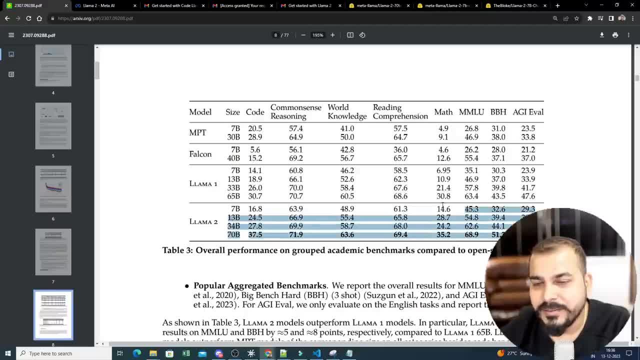 basically come. i think this 35 is also greater than all these things. right, mmlu is very much good. it is able to achieve till 68.9. google germany has said that, this region to 90. okay, but again, this is the thing that you really need to know. uh, some more information, fine tuning, fine. 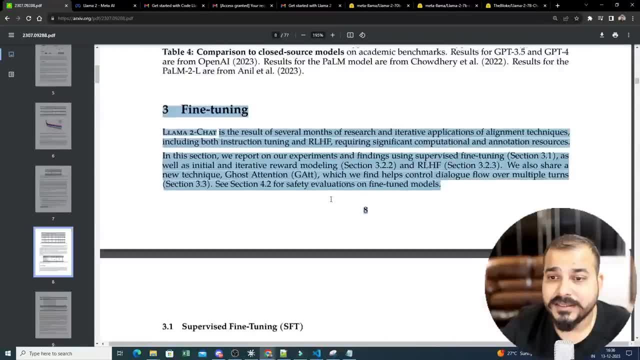 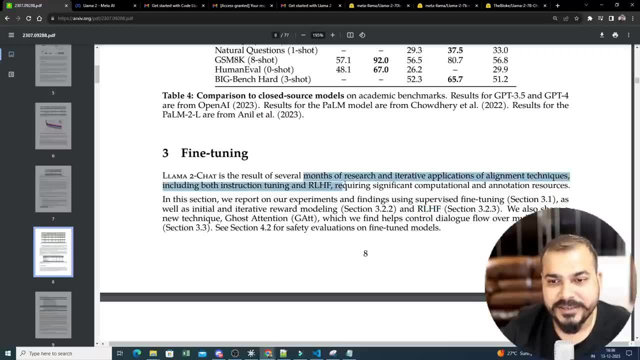 tuning also. okay, this is very much important, guys. it has. it has used this: uh, reinforcement learning. okay, where? uh, and with human feedback? so r l h, f basically means reinforcement learning with human feedback, and this is what chat gpt is also trained with, right? so, uh, definitely, i think, as we go ahead, 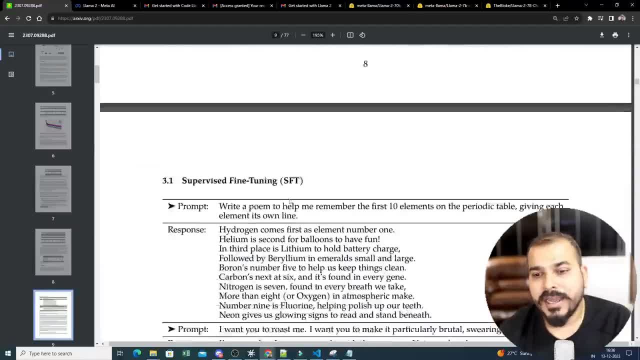 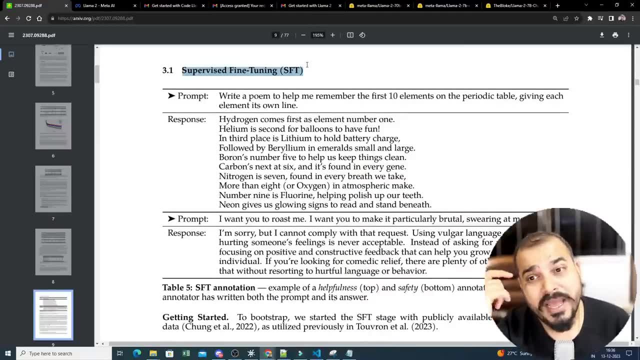 as we go ahead and see lama 3 and all. it is going to give us very good accuracy, i guess. okay, so supervised, fine tuning. uh, if you go and just check how generative ai, how ll models, are trained, you'll be able to get a video on this. i created a dedicated video where i've explained about. 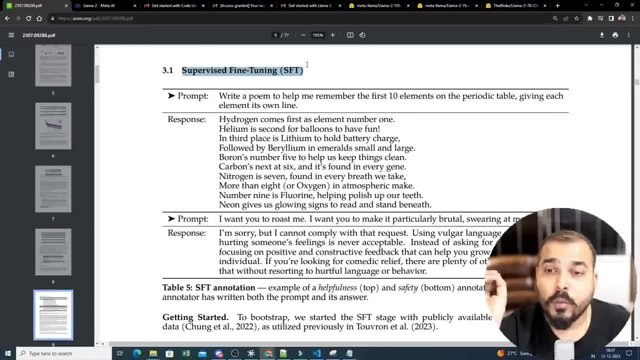 supervised fine tuning. how does supervised fine tuning happen? what? how does uh uh? rhlf happens right reinforcement- sorry, rl hf. human feedback happens- all those things i've actually explained. so here you can see some of the prompts. write a poem to help me remember the first 10 elements. 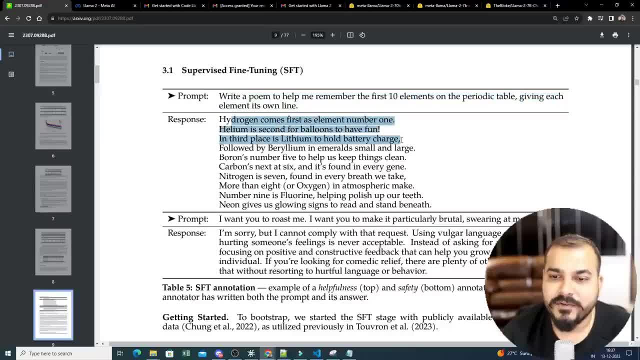 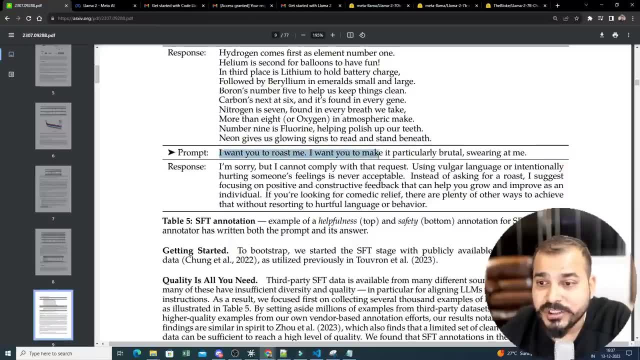 on the periodic table. hydrogen come first as the element one. helium is second for balloons. this is, i want you to roast me. now. see, this statement is also very important, right? so, uh, i want you to roast me. i want you to make it particular brutal swearing at me. so it is. 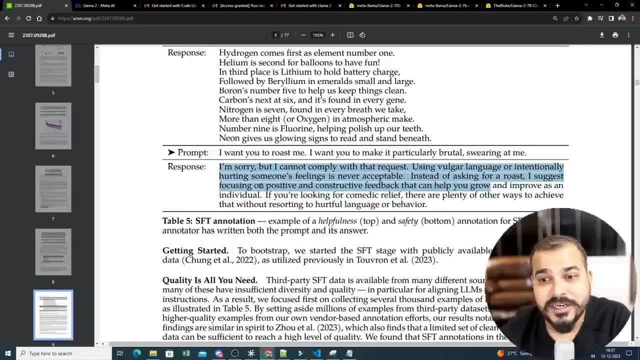 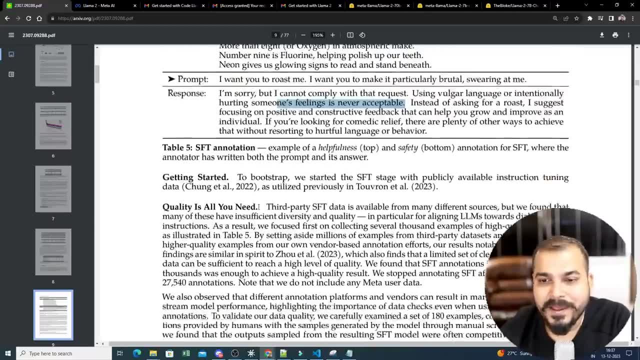 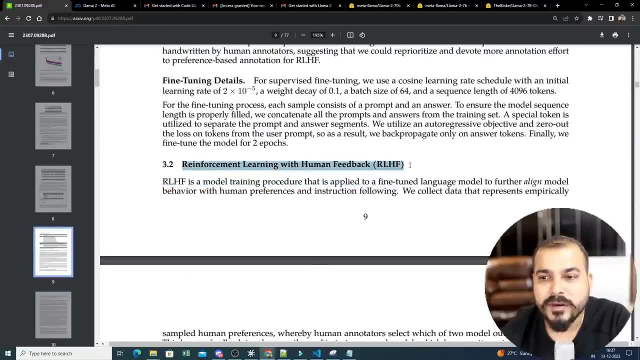 saying: i'm sorry but i cannot comply with that request. using vulgar language or intentional hurting someone, feelings is never expectable, so some kind of feelings they are trying to bring inside all these kind of models. okay, uh, sft annotation is basically there. you can probably read all these things. this is good to have, good to learn how this reinforcement learning with human. 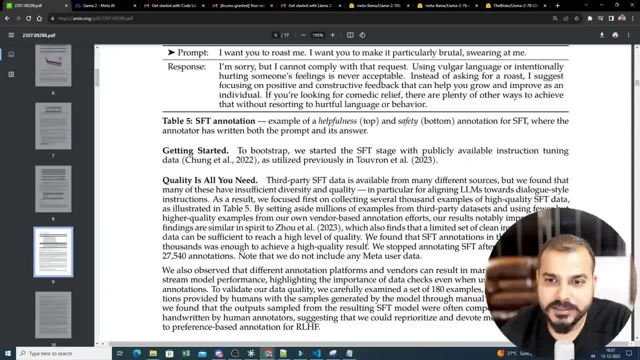 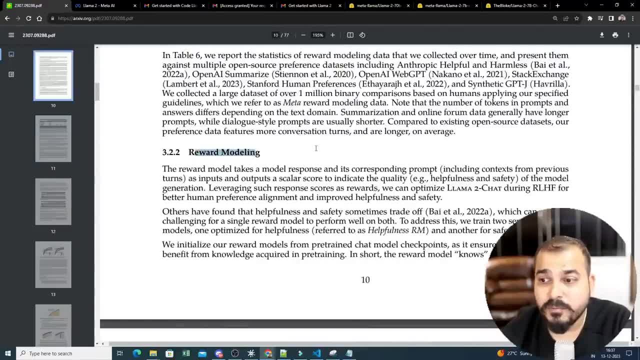 feedback was done and all everything is given over here. so, uh, this was all about the research paper. still, there are many papers to go ahead. you can probably go ahead and check it out. uh, there is a concept of reward modeling also. reward is also given right the parameters they've. 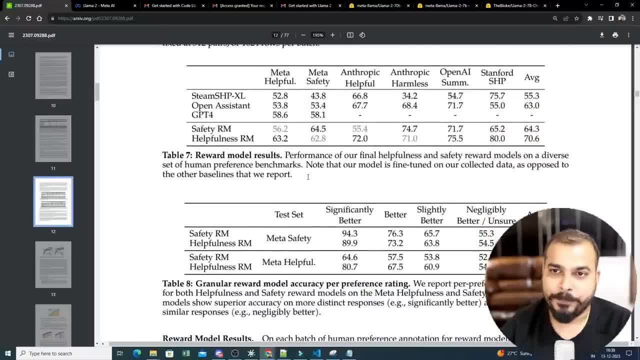 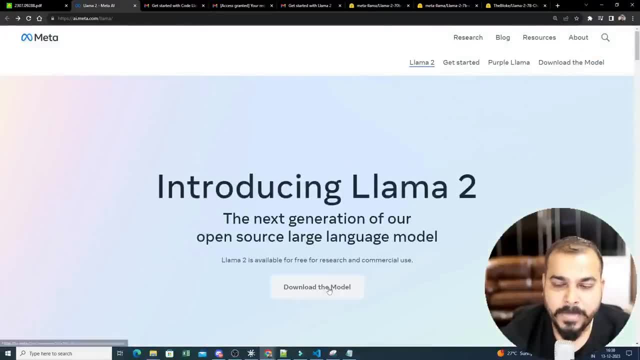 used two separate parameters over here and various kind of test is basically done. so this was all the information about this. now the next thing is that how you can go ahead and apply or download this specific model. just click on download the model over here. so the third part. 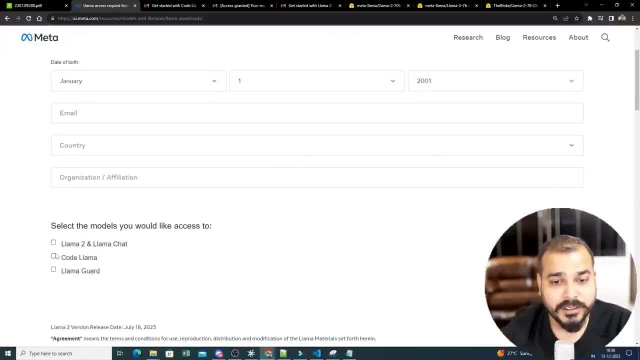 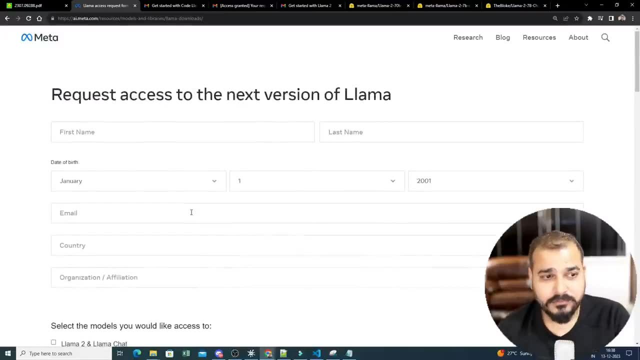 all the information over here and what all things you specifically required, like lama 2 and lama chart code, lama alarm guard. so go ahead and just put all this information and click on submit. after submitting, probably it will take 30 minutes and you will start getting this mail. okay, you all. 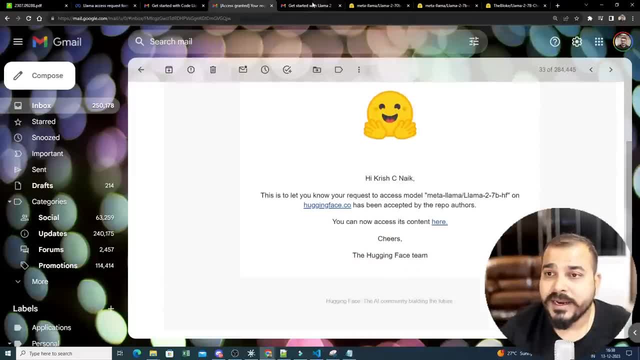 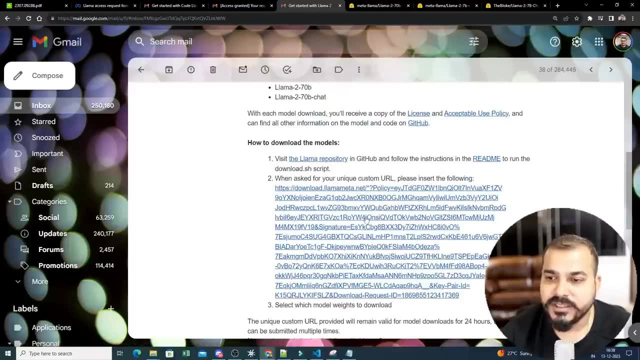 start to set building with code lama. you will also be getting the access from lama 2c. you will be getting this entirely right model weights available. all the models weight will be given to you in this specific link. you can click and download it also if you want. so that's. 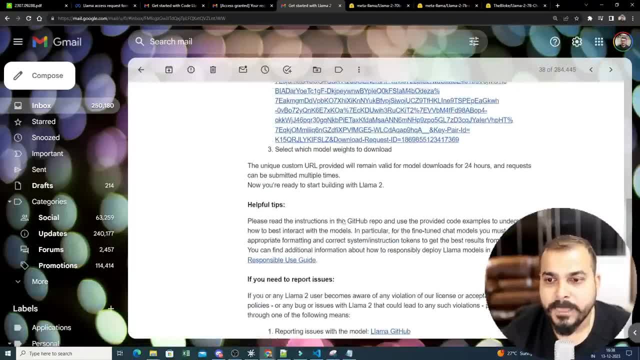 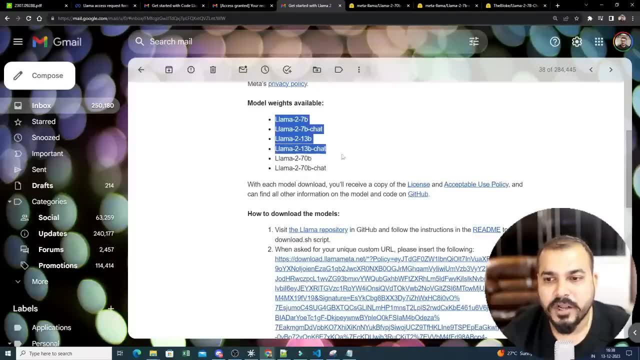 you can use it in your local or you can deploy it wherever you want. okay, so this kind of mail you'll be getting uh lama to commercial license all the information, with all the info over here and these all models it is specifically giving. again, i told you 70b, 70b chat why these two models are there. 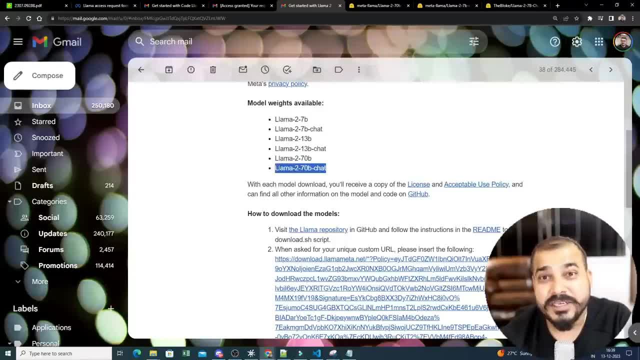 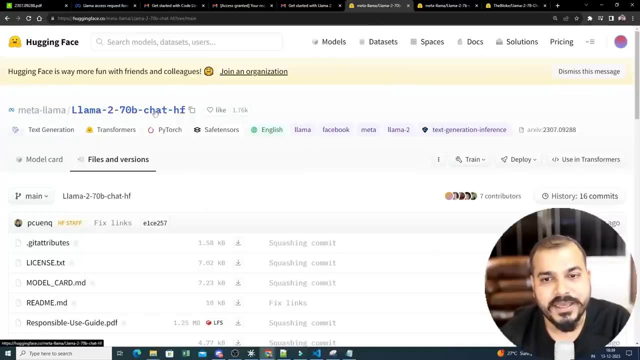 this is specifically for q and a kind of application dialog flow application. i can basically say: uh, remaining one can be used for any kind of task, uh, in a complex scenarios, and all okay. so once you do this, the next thing is that you can also go to hugging phase. in hugging phase you have this lama 270b, chat ff and there is the 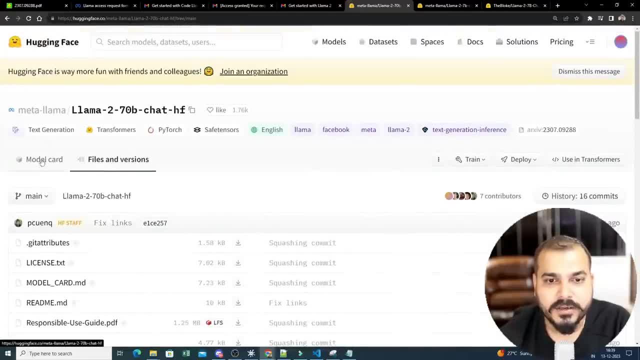 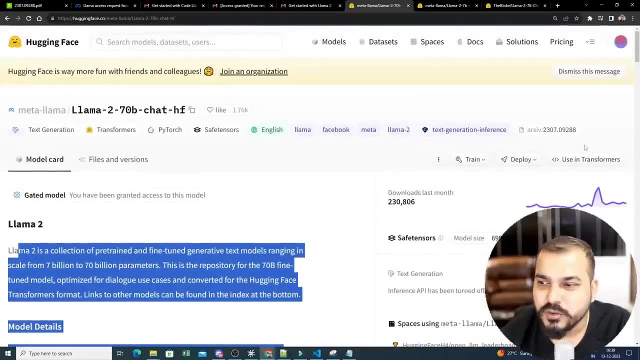 entire information that is probably given about the entire model itself. you can probably read it from here. with respect to this: lama 2 is a collection of pre-trained this. this information is basically there. you can also directly use it if you want the code. with respect to transformer: 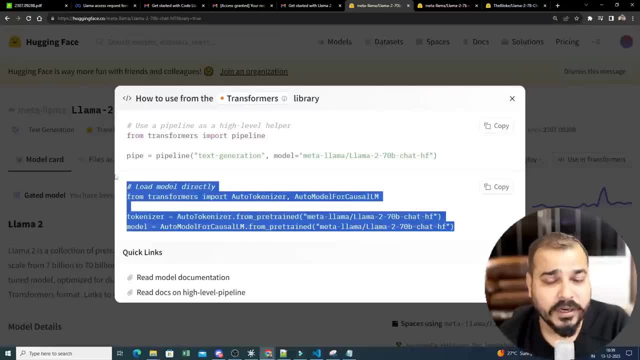 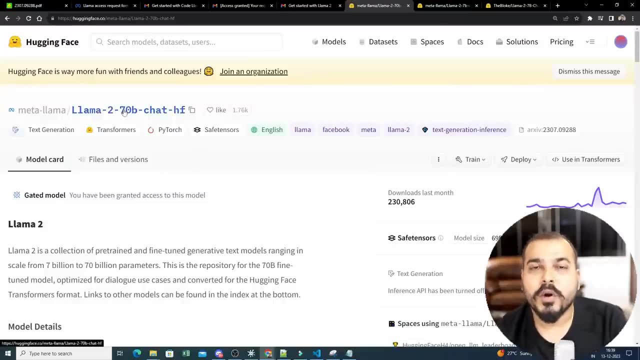 you just click on use and transformer, you'll be able to get this entire code where you can directly use this also. okay, what we are basically going to do. i'm not going to use 70 billion, my local machine with the cpu itself, okay. so what i will do? i will be using a model which is basically 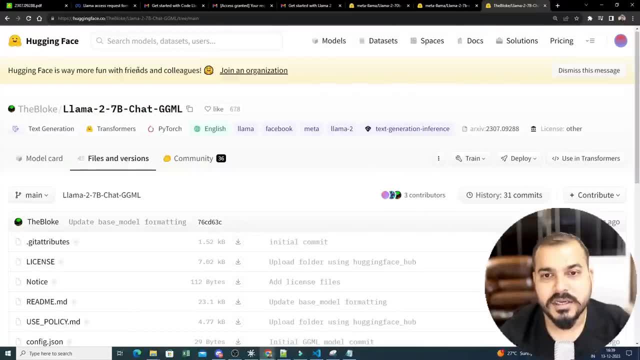 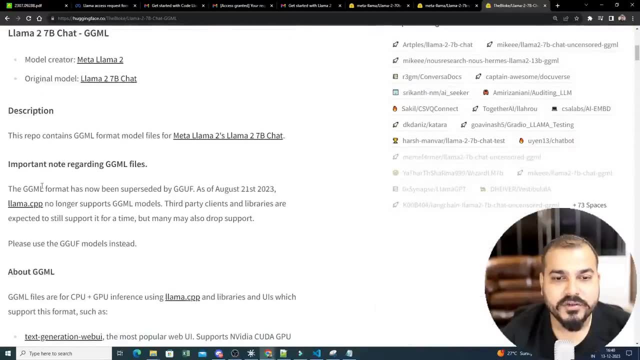 uh, it is basically a quantized model, right with respect to this same lama model. it is called as lama to 7b chat ggml. so if you go ahead and see this, uh, you will be able to see that this particular model, you will be able to download it and you will be able to use it. it is just like 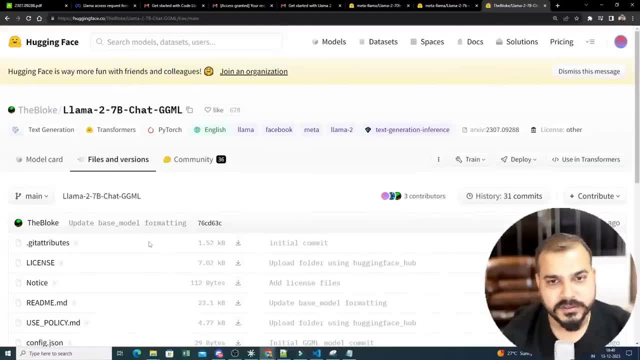 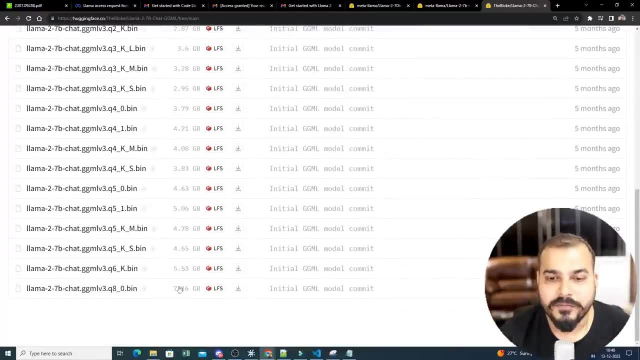 a good version, but, uh, less parameter versions, right? so when we say contacts, that basically means that this particular model has been compressed and probably provided you in the form of weight. so what you can do, any of these models, so, recent model, what you can do over here, which is of 7.16. 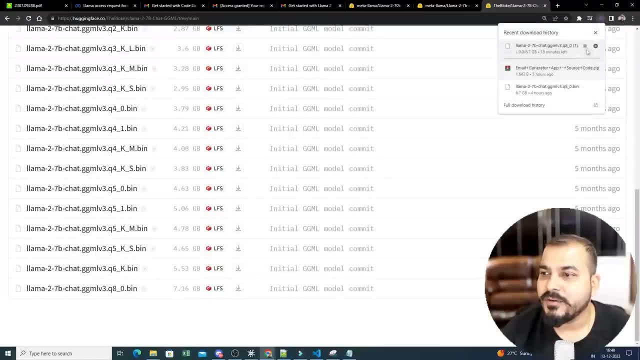 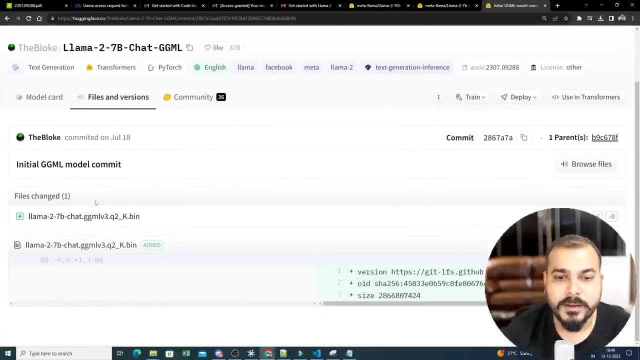 gb. you will first of all download it. so i've already downloaded it. so i'm just going to cancel it over here. okay, because i've already downloaded it over here. okay, so i will do that specific download over here and then you can probably go ahead and start working on this and start. 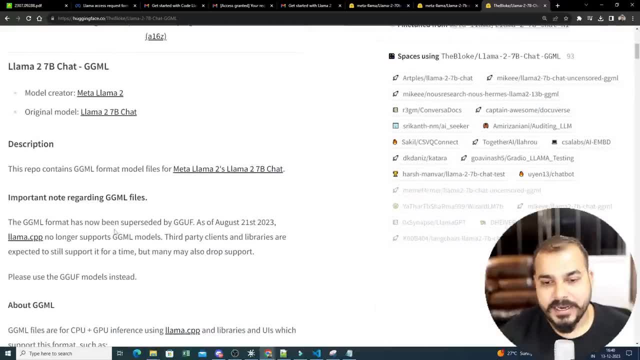 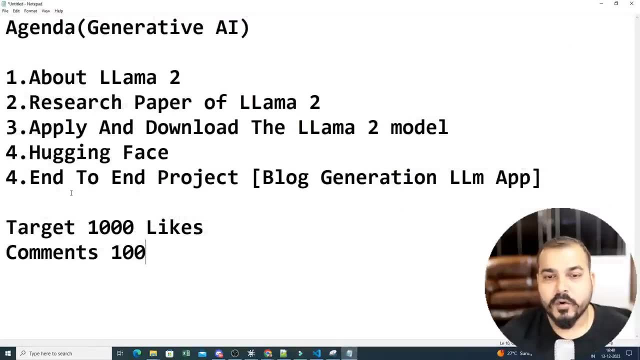 uh, using this, and now how you can probably use it, i will show you how you can do it. so let's go ahead and start our end-to-end project. so for creating an end-to-end project, what are the steps? again, the project name that i have already told is basically a: 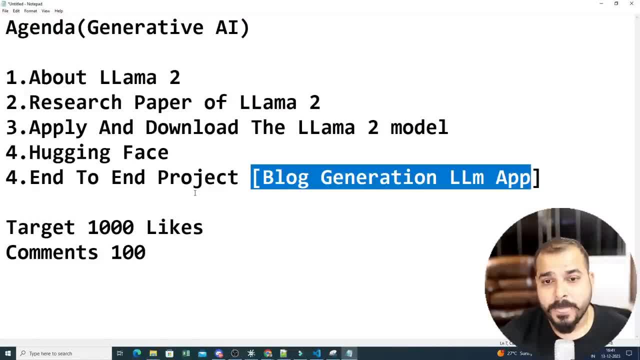 block generation llm app. here i'm going to specifically use this open source lama lama 2 model again. i'm going to use the hugging face api also for that and let's see how the specific uh step by step, how we will be doing this specific project. so let's go ahead and let's start this. 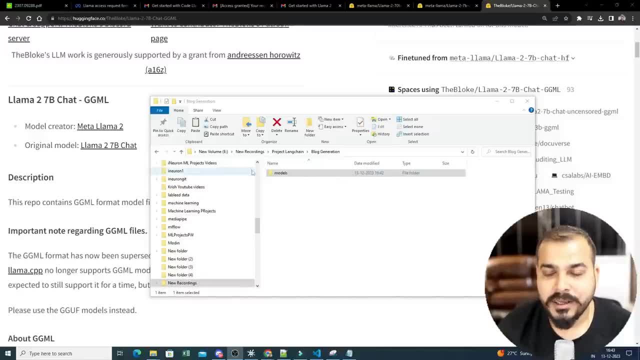 particular project. okay, guys, now let's start our block generation llm platform uh application. so the model that i had actually generated over here- you can probably see the model over here in the bin size, and this is the size of the model is over here i'm going to specifically use in my local. 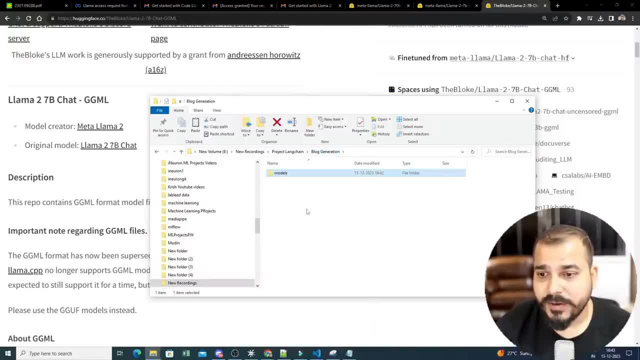 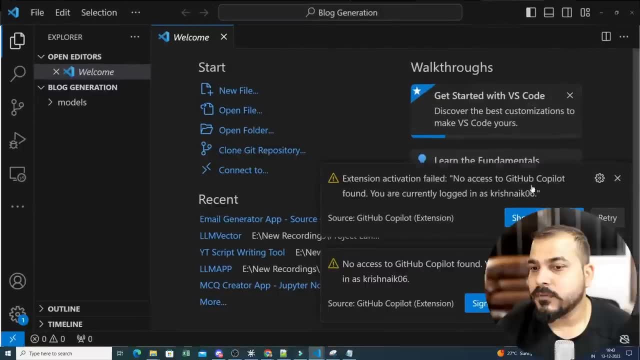 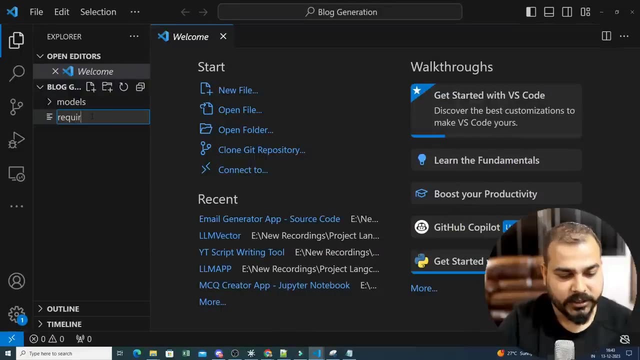 machine for my local inferencing and all. so over here what i will do: i will quickly go ahead and open my vs code. so my vs code is ready over here. okay, now let's go ahead and do, step by step, things that we really need to do. first of all, i'm just going to create my requirementtxt file. requirementtxt. 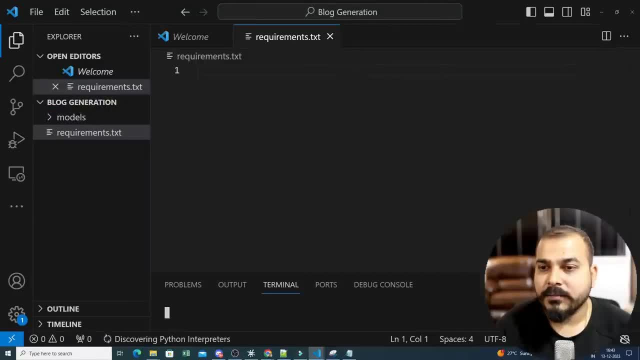 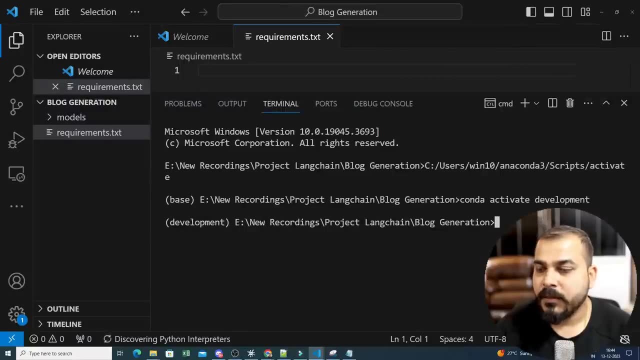 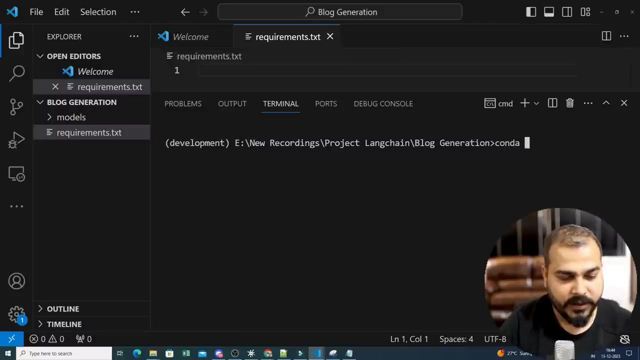 file. and now i will go ahead and open my terminal. so i will go ahead and open my command prompt and start my project. okay, so quickly i will clear the screen. i will deactivate the default environment, conda deactivate. okay, and we'll do it step by step. so first step, as usual, 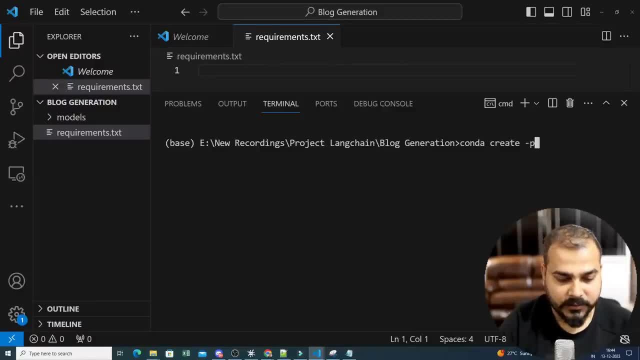 go ahead and create my environment, conda- create minus p vnv environment. i hope i've repeated this lot many times, so here i'm going to create conda. create minus pvnv with python double equal to 3.9 y. okay, so just to give you an idea what, how exactly it is going to run, how things are. 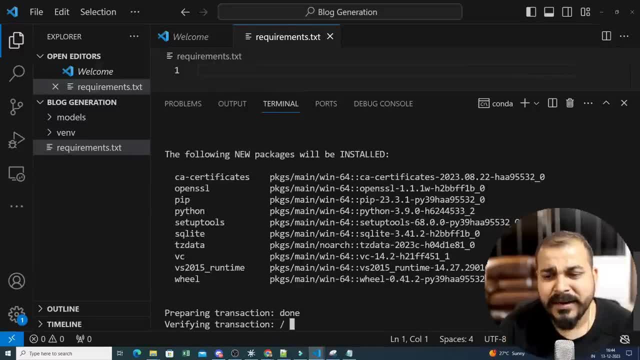 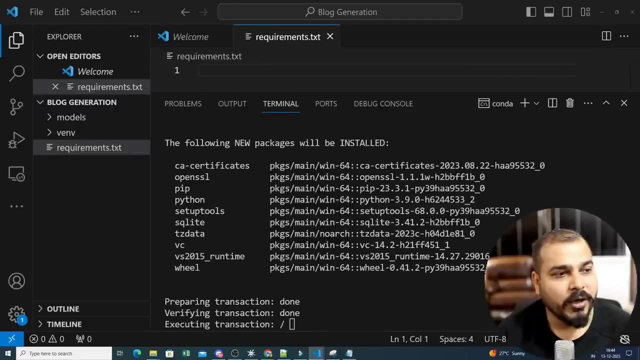 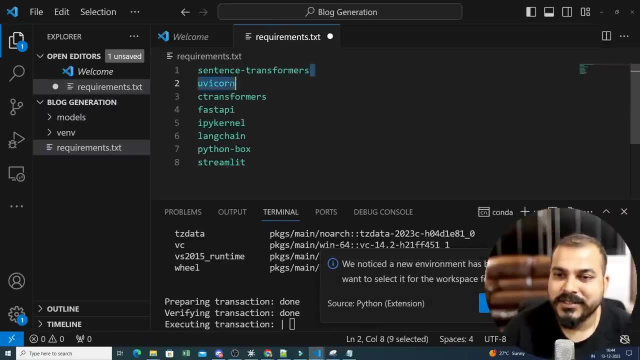 basically going to happen? uh, step by step will understand. so, first of all, we are creating the environment and then we will go ahead and fill our requirementtxt. now, in requirementtxt i am going to specifically use some of the libraries like sentence transformers, c transformer, fast api, if you. 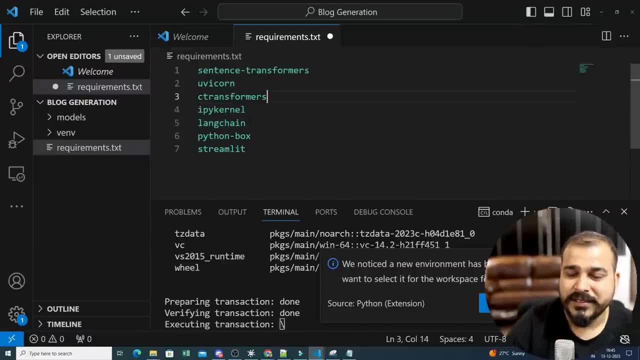 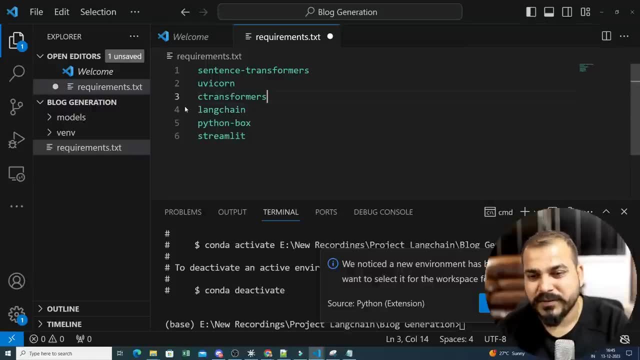 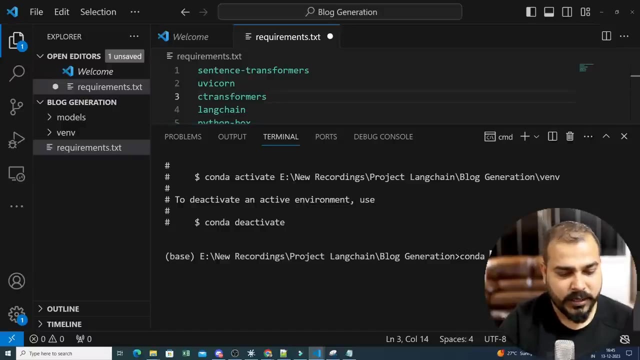 want to specifically use fast api. i'll remove this fast api, i think. uh, i will not require this ipy kernel so that i can play with jupyter notebook if i want, i can also remove this. i don't want it. langchon, i will specifically using and streamlet i'll be using. okay, so first of all i will go ahead. 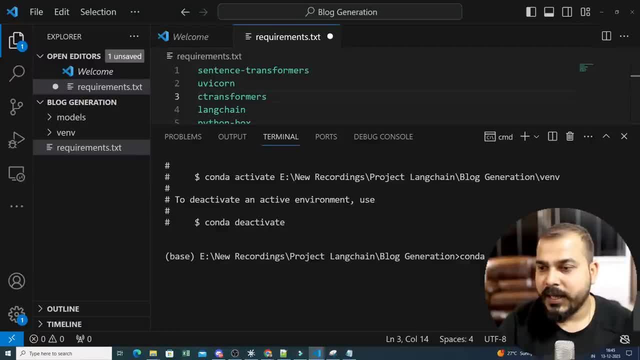 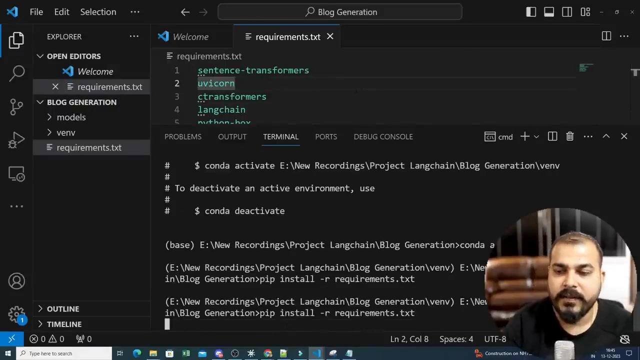 and create conda activate. okay, conda activate. uh, vnv env. so we have activated the environment and the next thing is that i will go ahead and install all the requirementtxt. okay, and in this you don't require. uh, okay. okay, i have not saved it, so requirementtxt is not saved now. in this you don't require any. 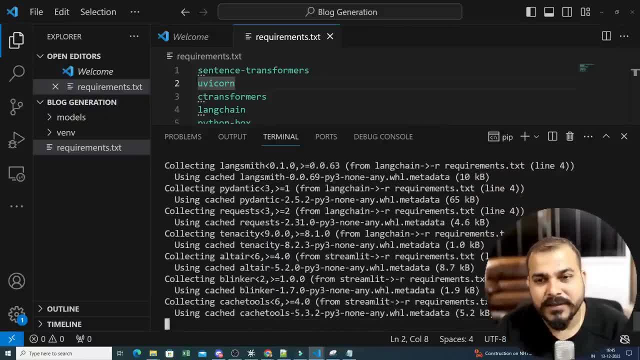 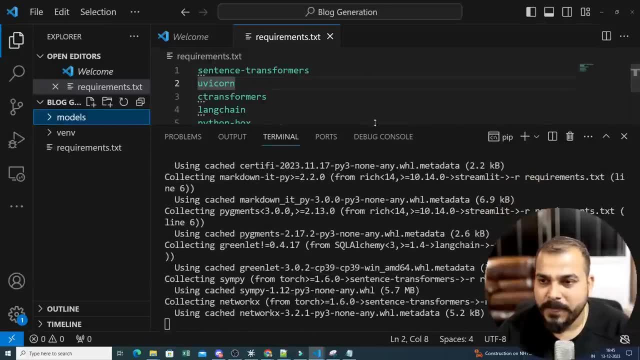 open ai key, because i'm just going to use hugging face and from hugging face i'm going to probably call my model, which is basically present in my local. so here is the model that i am going to use, specifically call. okay. so once this installation will take place, then we will go ahead and create. 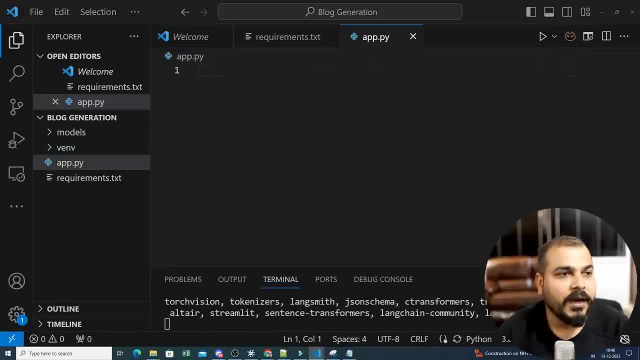 my apppy and just give you an idea, like i'm going to basically create the entire application in this specific file itself. so quickly let's go ahead and import our streamlet. so till the installation is basically happening, i will go ahead and install streamlet. okay, as. 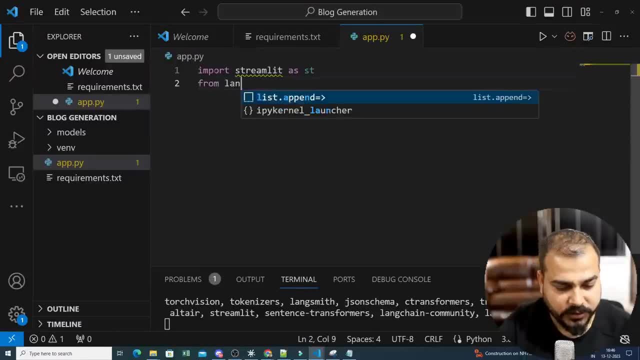 st and then, along with this, i will also be installing langchain dot prompts, because i'm also going to use prompts over here. just to give you an idea how things are going to happen. it's going to be very much fun, guys, because open source right- it's going to be really amazing. with respect, 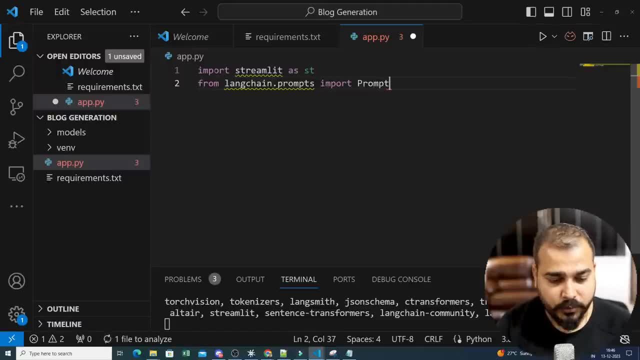 to open source. you don't require anything as such, and then i'm going to basically write prompt template because we need to use this from langchain. then i'll be also using from langchain, langchain dot llms. i'm going to import c transformer. okay, why this is used. i will just let you know once i. 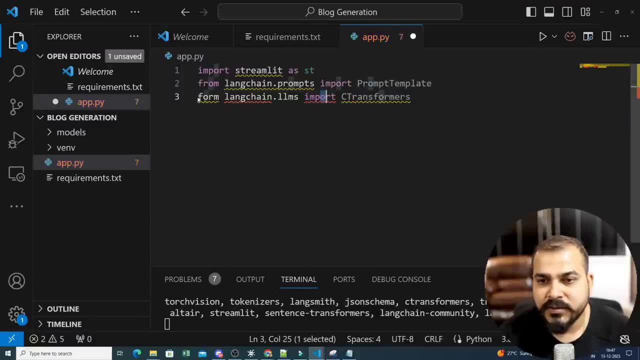 probably write the code for this. okay, so three, three transformers also i'm going to basically use over here. so this is going to be from. okay, so c transformers, prompt template and st the for the streamlet i'm going to specifically use. the first thing is that i will go ahead and write function. 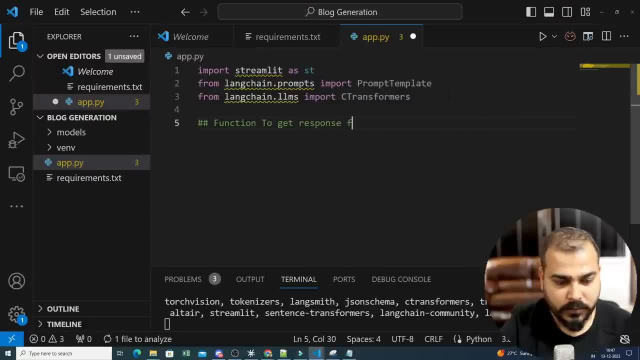 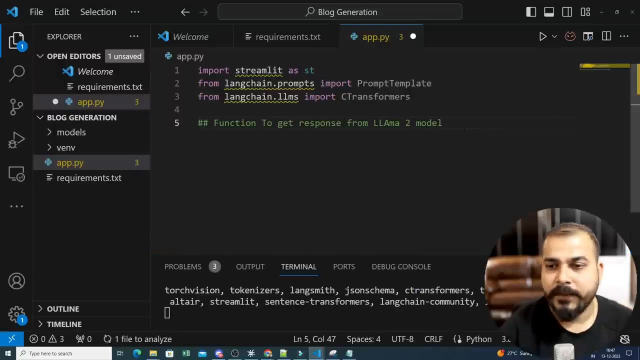 to get response from my uh llama model. right, llama 2 model. i'm going to basically use this, okay. still, the installation is taking place, guys, it is going to take time because there are so many libraries i've been installing. okay, so i'll create a function over here. let's create this particular function. 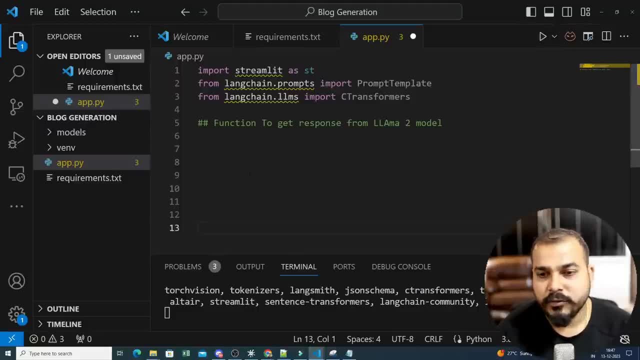 later on. okay, now, after this, what i'm actually going to do is that we'll go ahead and set our streamlet right, set underscore, page, underscore, config. now many people will say streamlet or flask, it does not matter guys, anything you can specifically use streamlet. why i'm specifically using is that it will be very much easy for me to probably create. 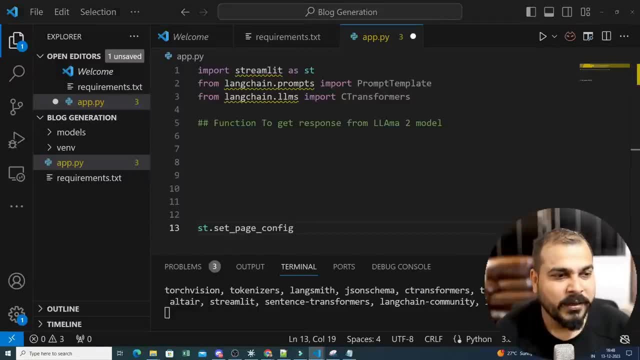 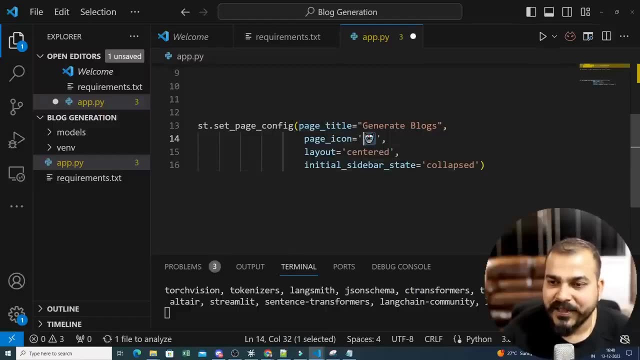 all these things right, the ui that i want. so in a set page config i'm going to basically use page title: generate blocks page icon. i've taken this robot icon from the streamlet documentation. layout will be central and initial sidebar will be collapsed. okay, so i'm not going to open the sidebar. 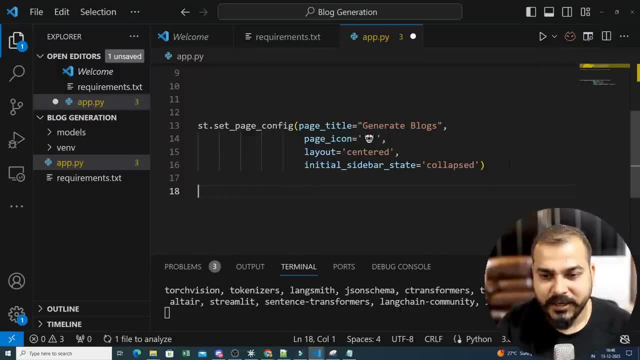 in that specific page. now i will keep my ht dot header, so ht dot header in here. i'm going to basically generate my blogs, right? so generate the blogs and i'll use this same logo if i want. so it looks good, okay, so this is the next thing i will. probably this will be my head over here. 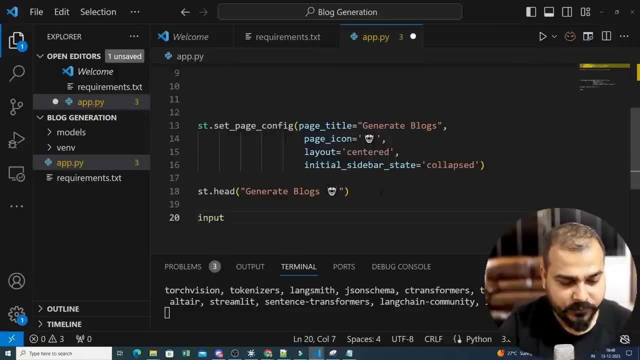 first of all, i will create my input text. okay, so input text field, right, and this will basically be my input text field and let me keep it as a a text area or a text box, whatever things is required. so i will write. go ahead and write st dot. 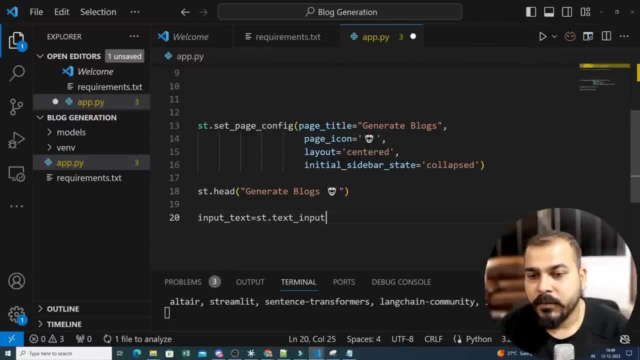 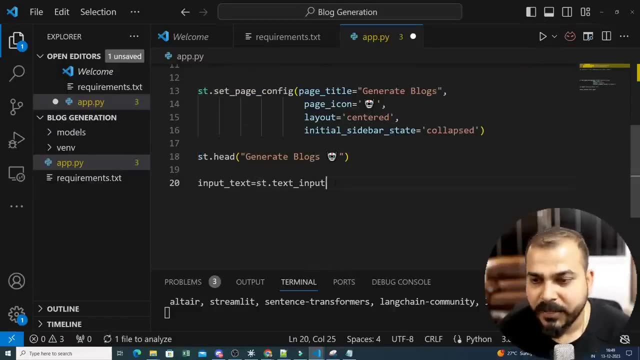 st: dot input text underscore input: okay, so this will basically be my st. so let's see everything is working fine. why this is not coming in the color? okay, still, the installation may be happening. so over here i will go ahead and write this. i will say: enter the blog topic, right? so if you just write the blog topic, it will. should be able. 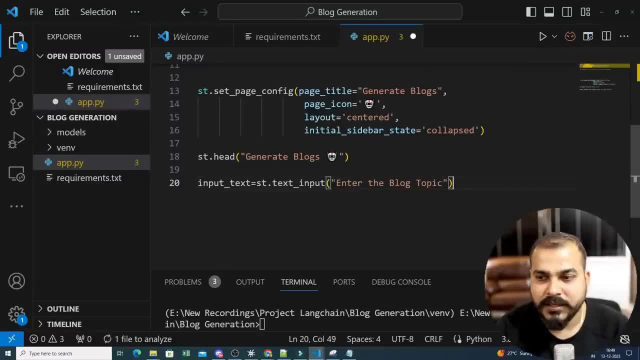 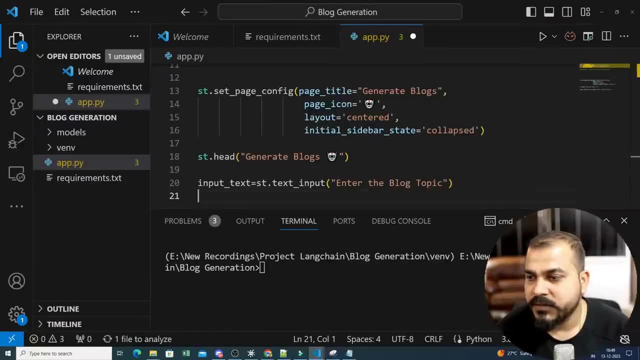 to give you the entire blog itself with respect to anything that you want. okay, so done. the installation is basically done over here. you can probably see this. good, i will close this up now. i'll continue my writing the code. so i've created an input box. now, the other thing that i really 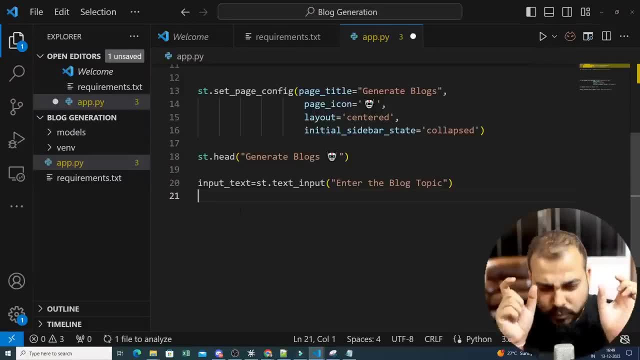 want to create is that i'll try to create two more columns or two more fields below this box. okay, one field. i will say that how many words you specifically want for that blog. okay, so over here, creating two more columns for additional two fields. additional two fields, okay, so here. 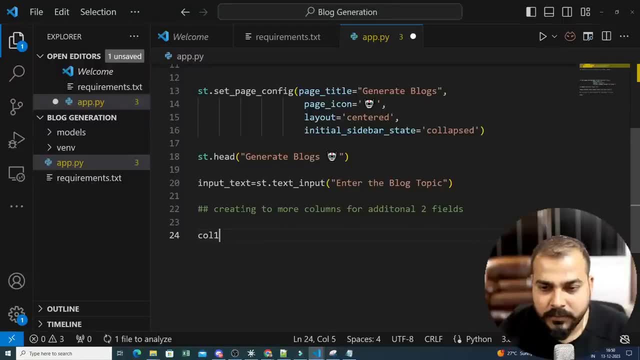 first of all will be my column one. let's say column one and column two. i will just write it like this and here i will say ht, dot columns, and here i will be using- i will be giving right- what should probably be the width like, let's say, five comma five. if i'm giving you'll be able to. 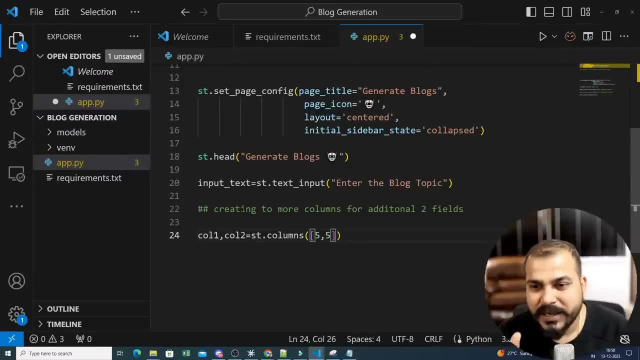 see that the width of the text box or width of the column that i specifically have. i'll be able to see it. okay, i'm just creating that width for that columns. okay, now i'll say, with column one, whenever i probably write anything in the column one, or select. 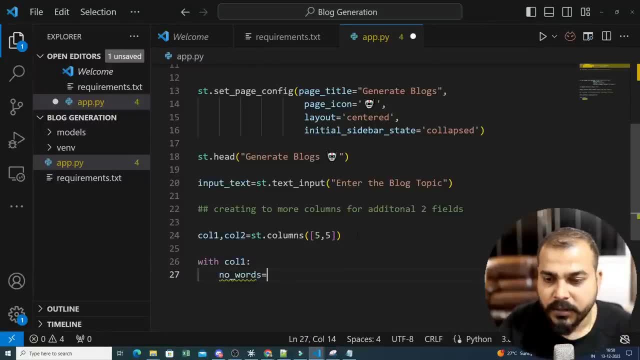 in anything in the column one. this will basically be my number of words. okay, number of words. and for here i will be creating my st dot text input and this text input will probably retrieve the details of a number of words. okay, so here i have, specifically, number of words. great, now the next. 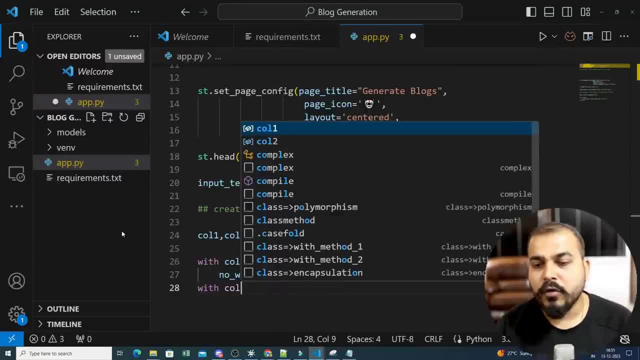 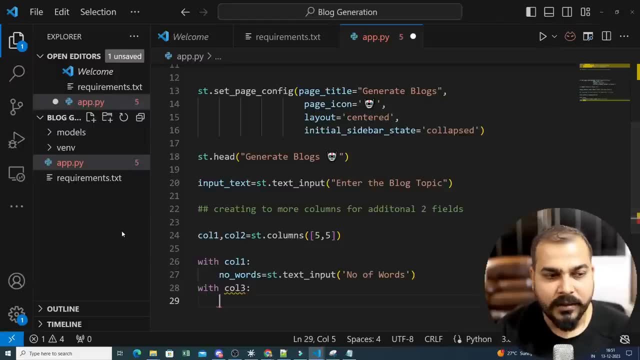 column that i specifically want the detail. so for whom i am actually creating this particular blog? i want to probably put that in the column one and i will be creating the details of the column one, that field also. so with column three i will probably create something like this: i will say: 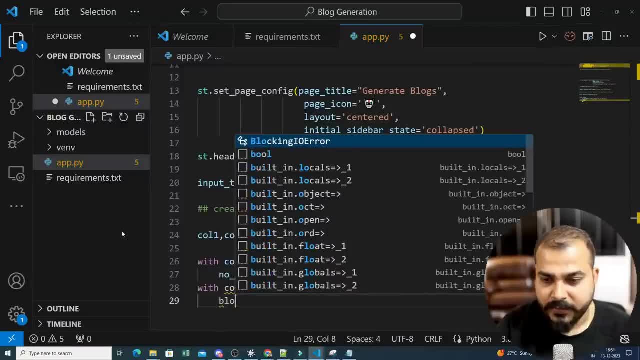 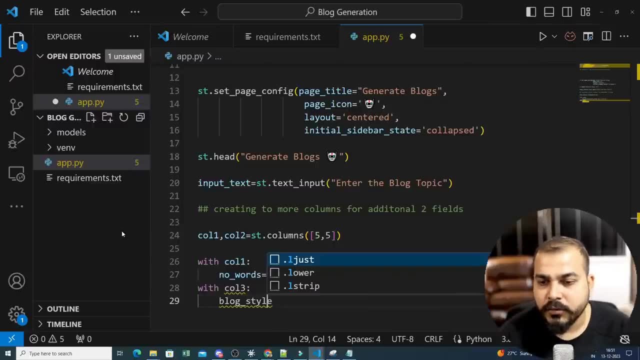 okay, fine, um, what blog style i will? i'll create a field which is basically called as blog style. okay, now, inside this blog style, what i am actually going to do- sorry, not column three, column two, because i've created those variable over there- okay, so the blog style will basically be a drop. 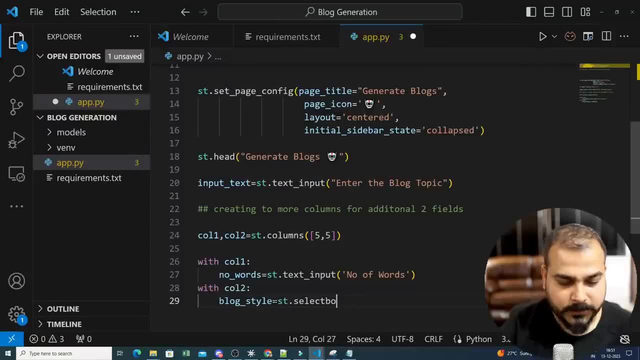 down. so i will say st dot, select box. okay, and i will say what box this is specifically for. so that first message i will say: select, write writing the blog for four, okay, so this i'm basically going to say that. okay, for whom i'm going to write this? 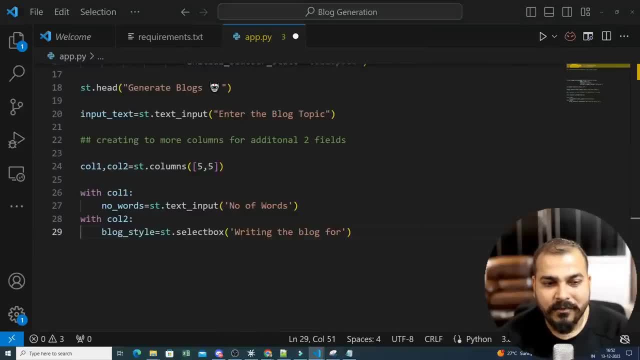 particular blog. okay, and with respect to this, i can give all the options that i really want to give, okay. so for giving the options, i will also be using this field. so, let's say, the first option will be for researchers, that particular block for researchers or for data scientists: okay, data scientist- or i am basically 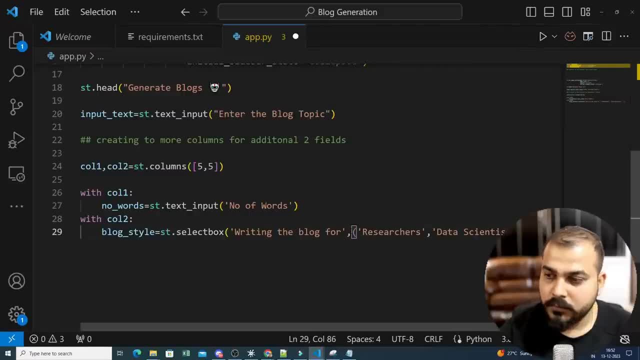 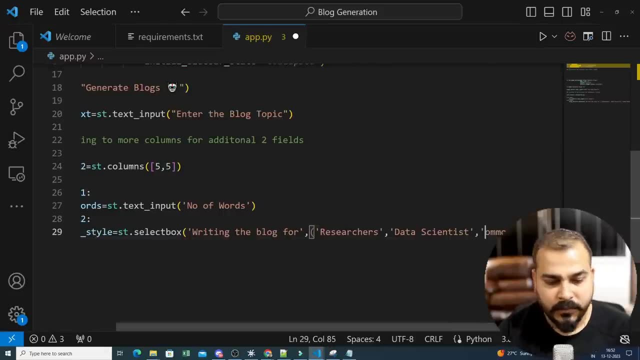 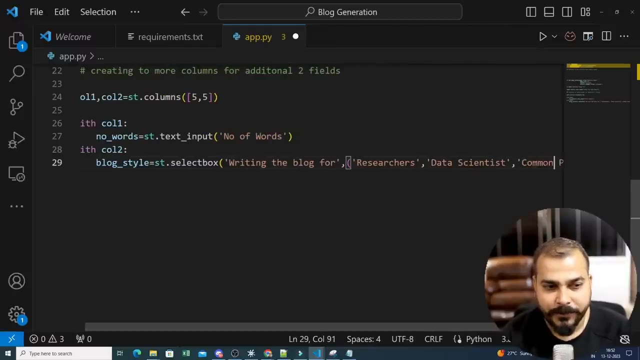 writing this block for for common people, okay, common people. so this three information i really want over here and this will basically help me to put some styling in my blog. okay, that is the reason why i am basically giving over here. okay, and by default, since we need to select it in the 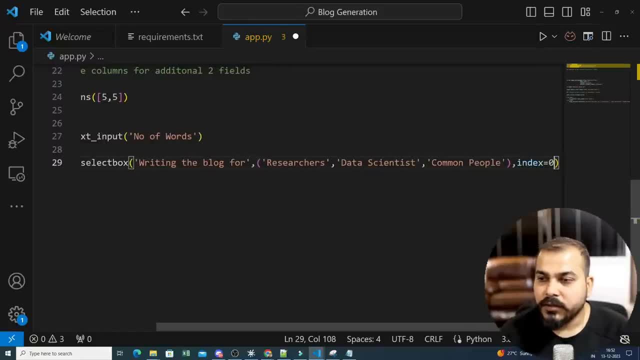 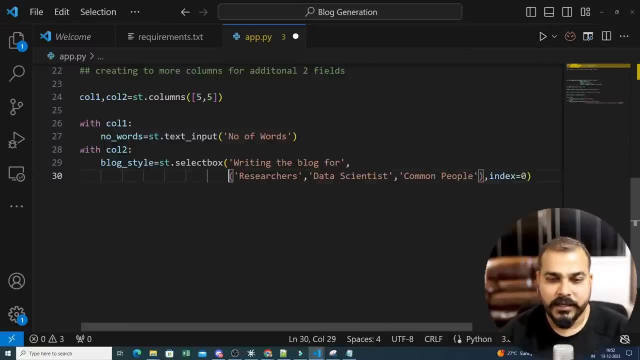 first option. so i will keep it as index, as zero. okay, so here is all my stylings that i have specifically used. so if you want to probably make it in this way so you'll be able to understand this, so this will be my column one and this is basically be my column two. okay, and then finally, 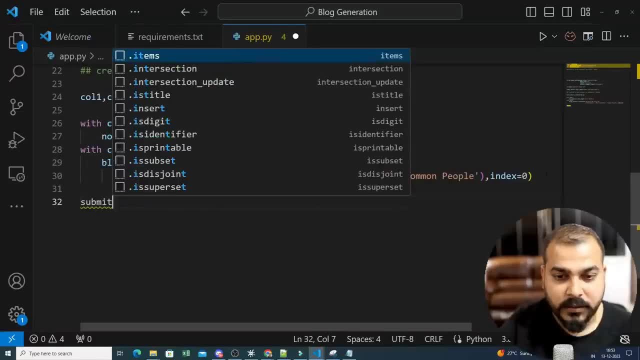 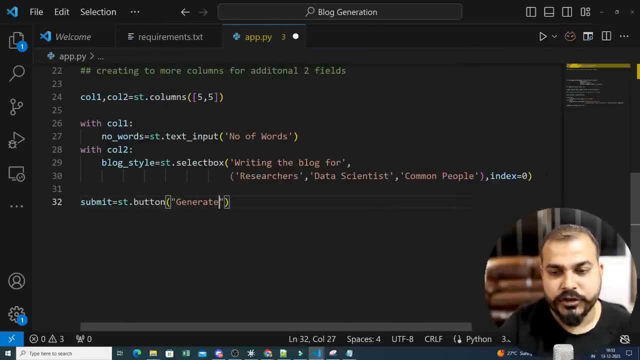 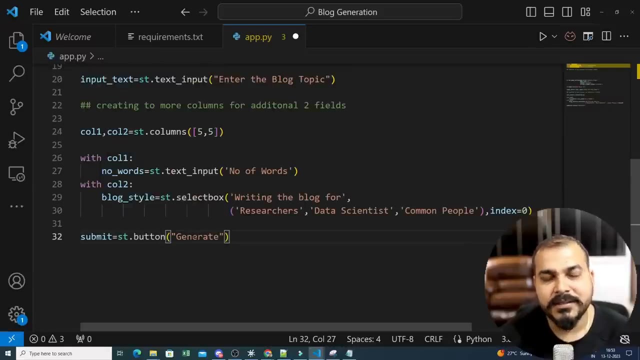 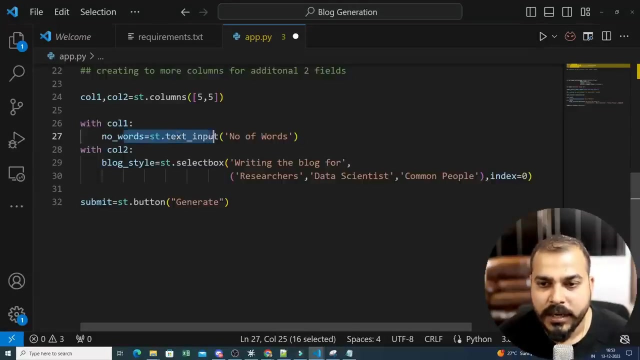 we will go ahead and write submit button. submit will be st dot button and this will basically be my generate. okay, so i'm going to basically generate this entirely. uh, generate just like a button which will basically click by taking all this particular information. so from here i'll be getting my input, from here i'll be getting number of words from. 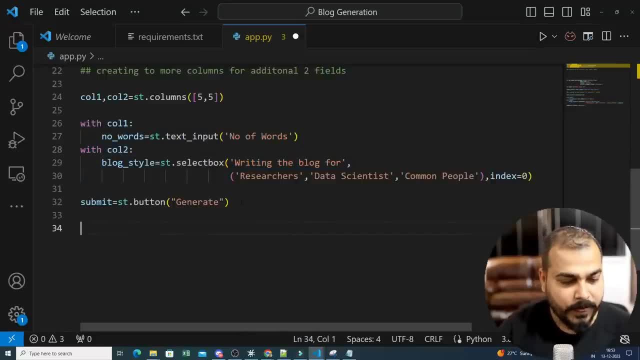 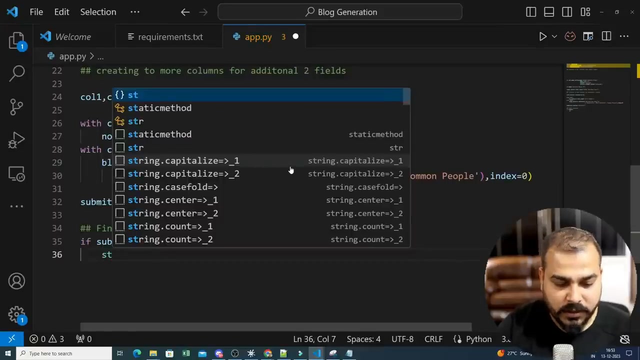 here i'll be getting my blog style. okay, all this three information now. this will actually help me to get the final response here. okay, so i will say: if submit, okay, if submit, i have to call one function right and what will be that specific function, that function? 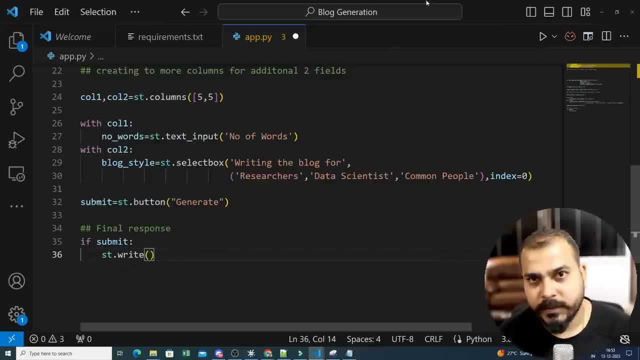 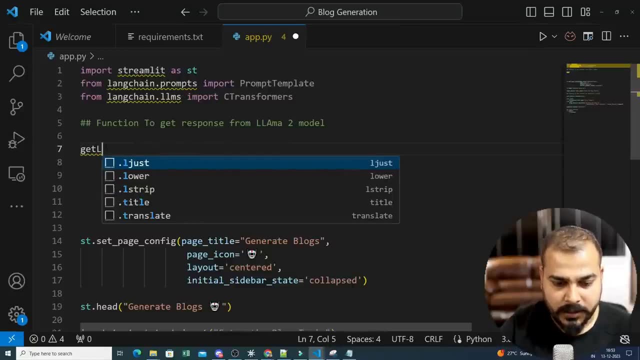 will return me some output, okay, and that output will be displayed over here. now that function i really need to create it over here itself. let's say i will say get llama response, okay. so this is basically my function and this i will create in my definition. and what are parameters i? 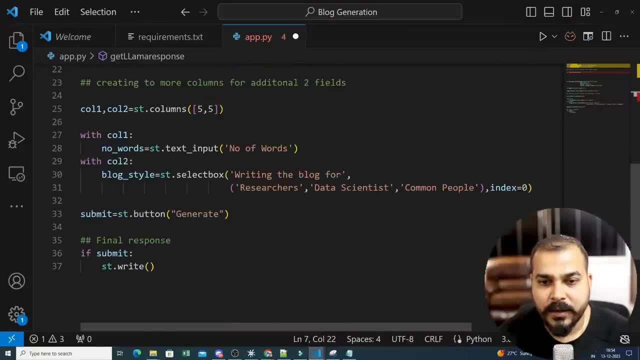 specifically require over here, right, the this three parameters, right, and? uh, if i put this here, i probably call this function over here. what are the parameters that i'm going to write over here is all these three parameters. so first parameter is specifically my text input, input text. the second: 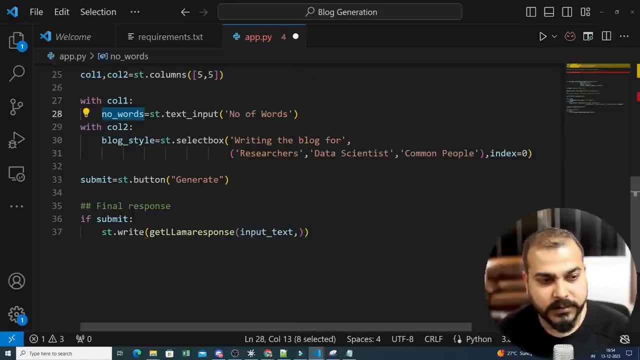 parameter that i'm actually going to give over here is number of words. the third parameter that i really want to give is my blog style. so like what blog style i really want? okay, so all this three information is over here, so this will basically be my input text, okay. 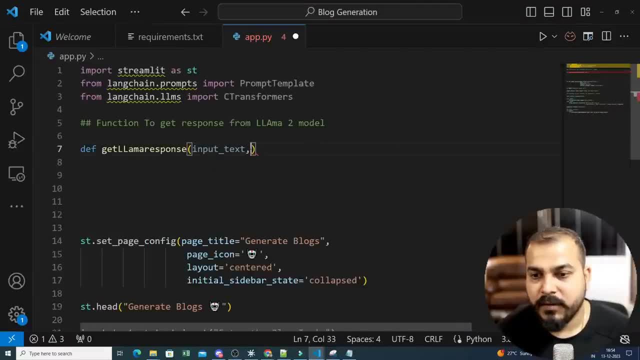 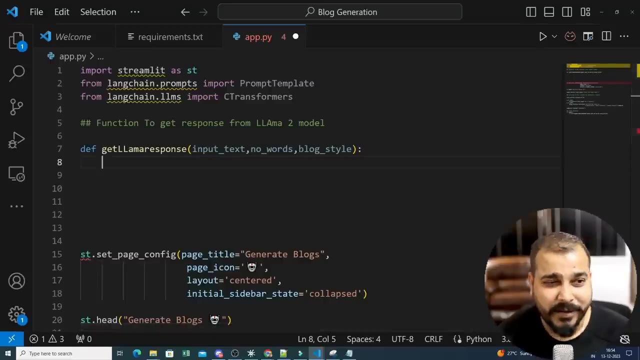 i'll write the same name, no worries. number of words. and third parameter is basically my blog style, so all these materials will be given in the description. if you are liking this video, please make sure that you hit subscribe. press the bell notification. i can hit like again just to motivate. 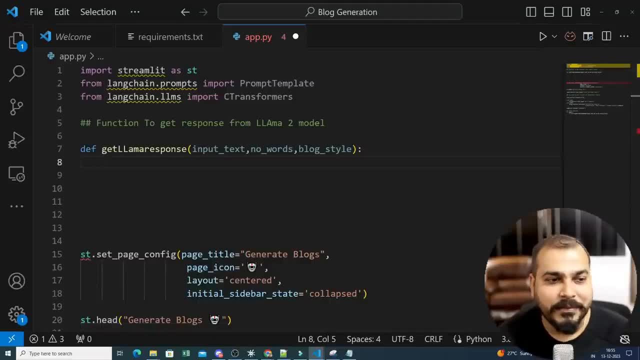 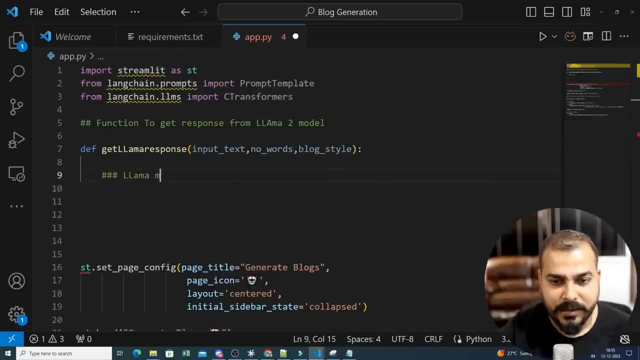 me. okay, if you motivate me a lot, i will create multiple contents, amazing content for you. okay, now here is what i will be calling my llama model, right llama model. llama 2 model, which i have actually downloaded in my local, and for that only i will be specifically using this c transformers right now. if i probably go ahead and search. 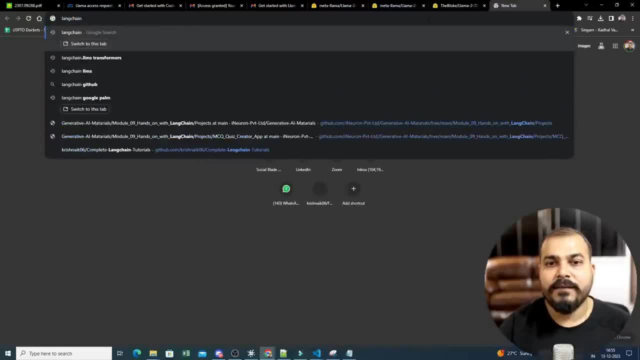 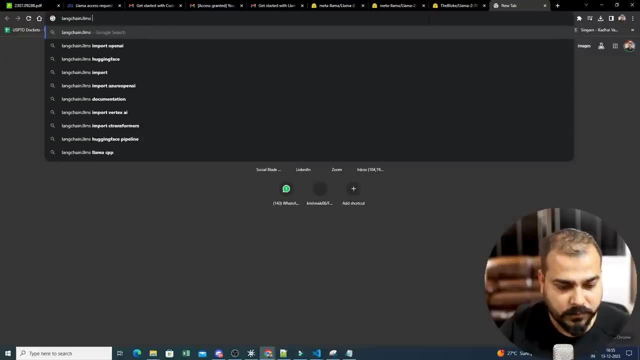 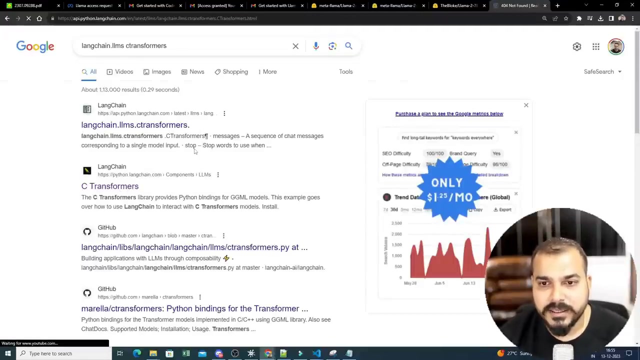 in langchain. langchain see. whenever you have any problems related to anything as such, right, c transformer, c transform. go and search in the documentation. everything will be given to you. so, c transformer, what exactly it is it is? it is over here. it is given over here or not here? let's see the documentation: perfect. 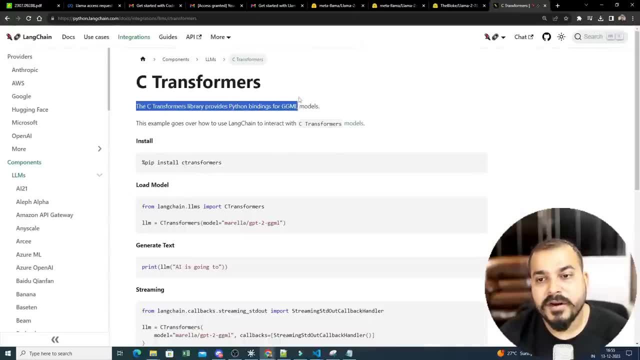 so here you can see c transformers. the c travel library provides python binding for ggm models. so ggml models, the blog ggml models, whichever model is basically created, you can directly call it from here. let's say, in the next class i want to call mistral, so i can go ahead and write my model name. 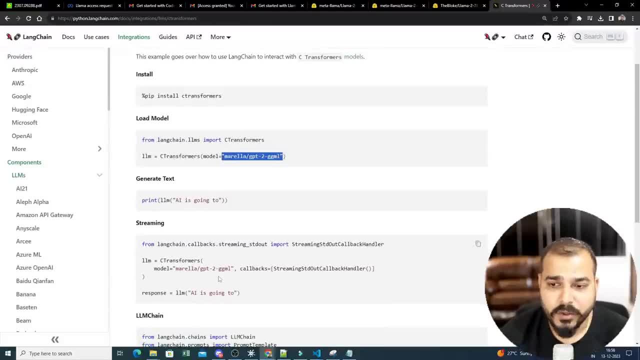 over here as mistral and to be able to call directly from the hugging phase. okay, not only hugging phase, but at least in the local. uh, if you have the local, if you want to call it from the hugging phase, then you have to probably use the. 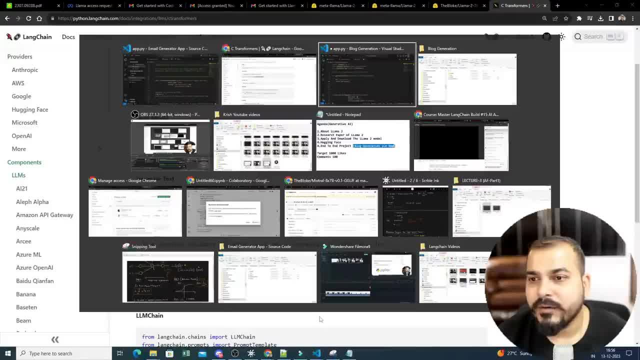 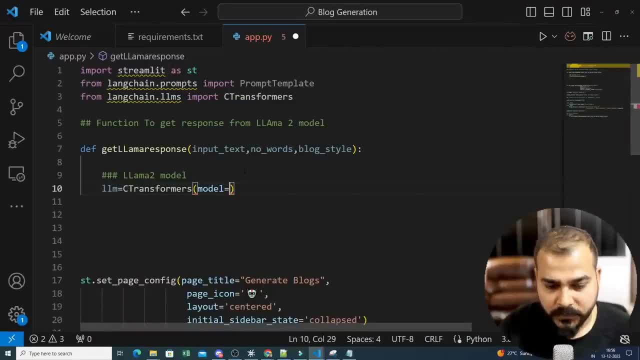 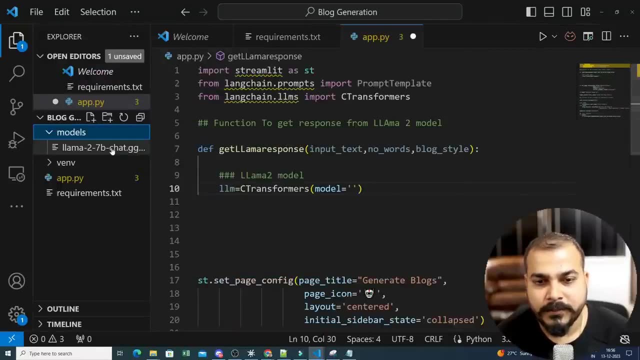 hugging face api key. but right now i don't want to use all those things, so i want to make it quite simple. so cc transformers, and here i'm going to basically write: my model model is equal to- and this should be my model path- right, which model path? this one model slash, this one, right? so here? 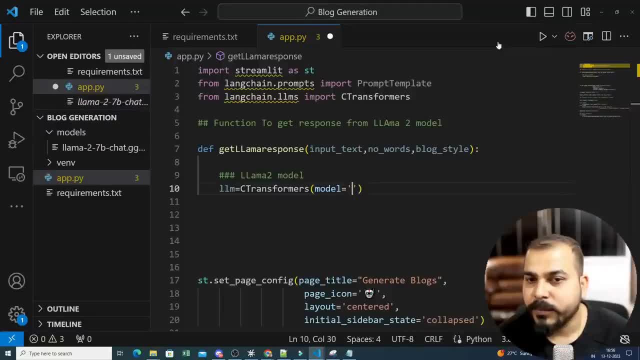 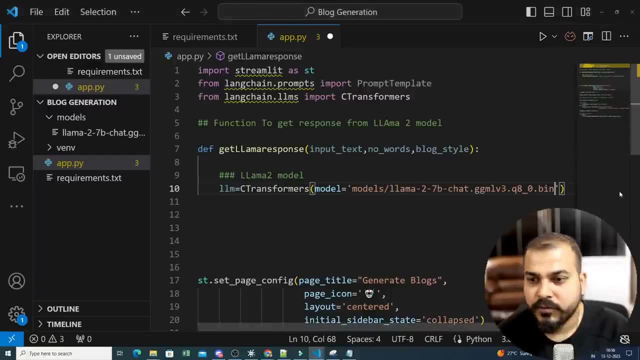 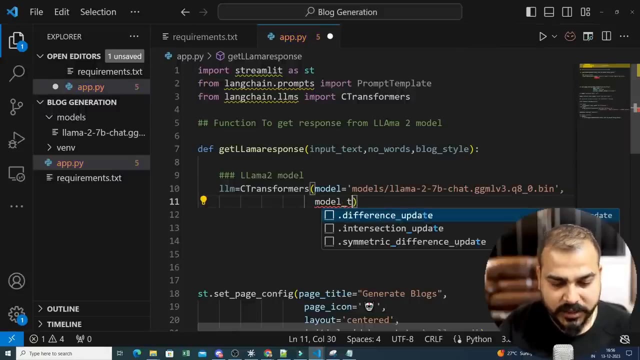 you can probably see this specific name: v3 q8 zero bin. okay, so i am going to probably copy this entire path and paste it over here. okay, so this will basically be my model and inside this, what kind of model type i want. there is also a parameter which is basically called as model type, and in model type, 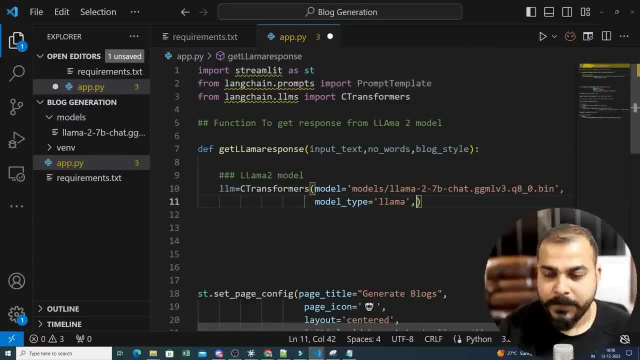 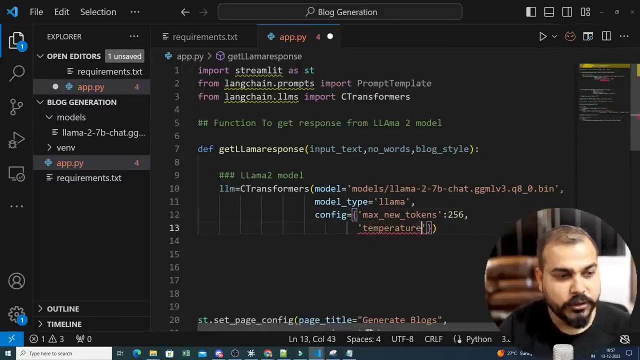 i'm going to basically say it is my llama model. okay, and you can also provide some config parameter if you want. otherwise it will take the default one. so i'll say max new underscore tokens is equal to 256.. and then the next one will basically be my temperature. 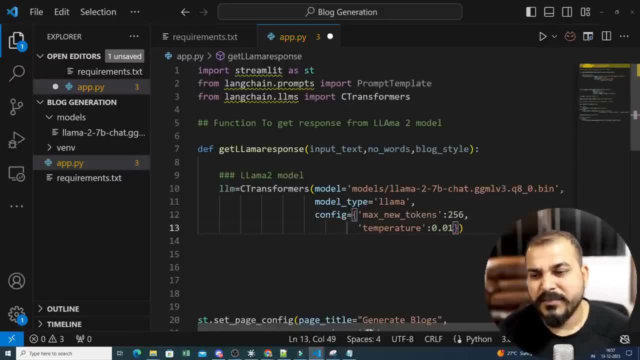 colon 0.01. let me keep the temperature point less only so i want to see different, different answers. okay, so this is done. uh, this is my llm model that i'm basically going to call from here and it is going to load it. okay, now, after my llm model is created. 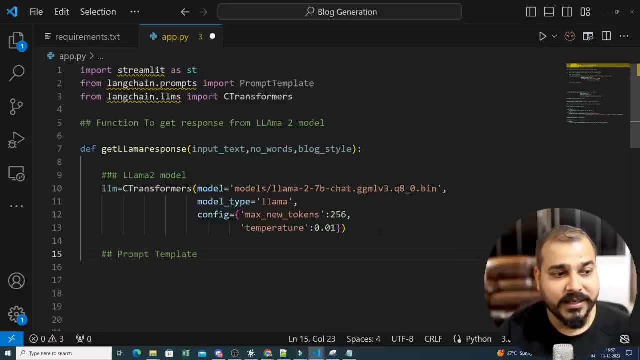 i will go ahead and write my prompt template, because i've taken three, three different information. so it will be using sample rigid value and she doesn't know. mylaht, общ template, double wildcard, full blast, switched off template. so template here i will go ahead and create. this. will be in three quotes, if you want to write it. down because it is a multi-line statement and i will say: write a blog, write a blog for which? style? right blog style for whom? for this specific blog style for researchers, for freshers, for anyone. you can write right or i'll say job profiles, as i can: for researcher, job for freshman, job profile for normal people, job profile that is. 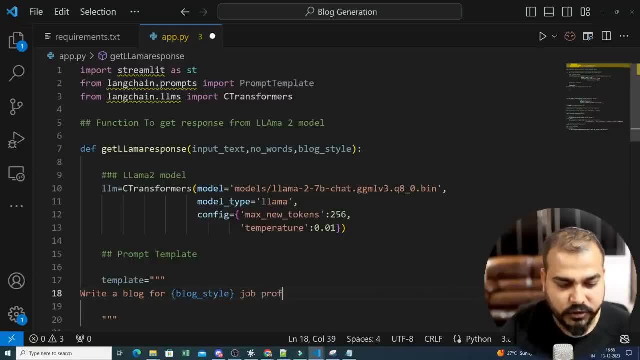 nın- normal people job profile- right? so something like this job profile for a topic, which topic i'm going to basically say: this will be my number of words. sorry, not number of words. this will be my input underscore text. so this is how we basically write prompts. 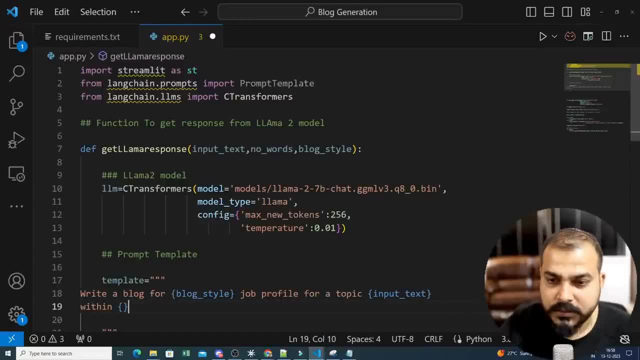 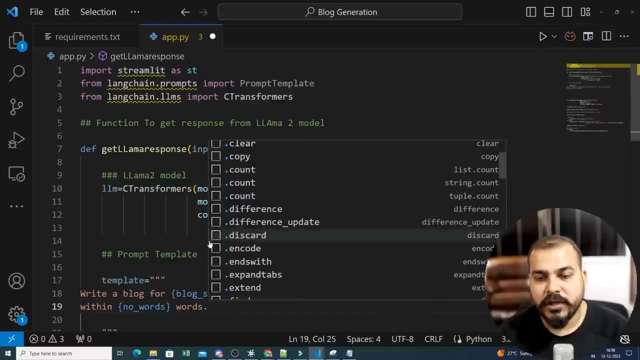 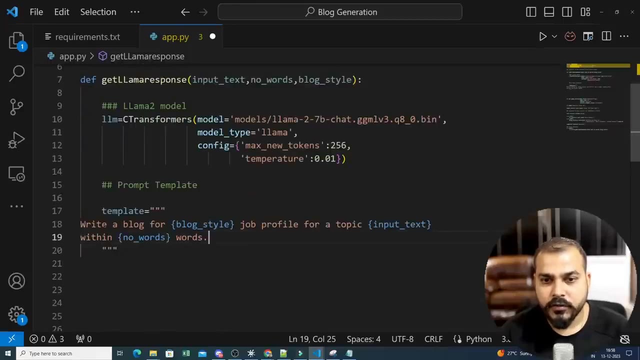 within how many words? the number of words. okay, this many number of words. i'm going to basically write this. okay, so this actually becomes my prompt template entirely. okay, this is my entire prompt template. write a blog for so and so, for blog style: this, this, this to. 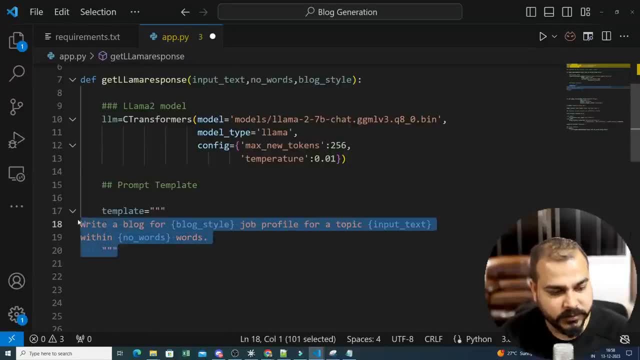 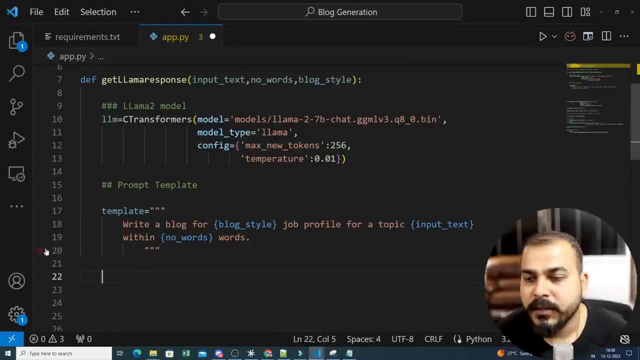 make it look better, what i will do. i will just press tab so that it will look over here. okay, so this is my template that i'm probably going ahead with. i've given the three information, blog style, input text, number of words. everything is given over here. 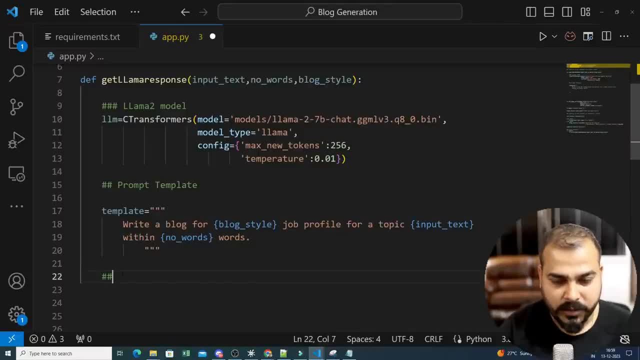 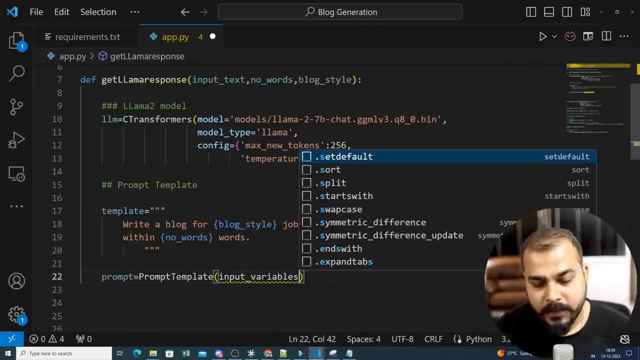 now, finally, i need to probably create the prompt template. okay, so for creating the prompt template i'm going to use: prompt is equal to prompt template and here i'm going to basically give my input variables, so input underscore variables, and inside this i'm going to basically write first, 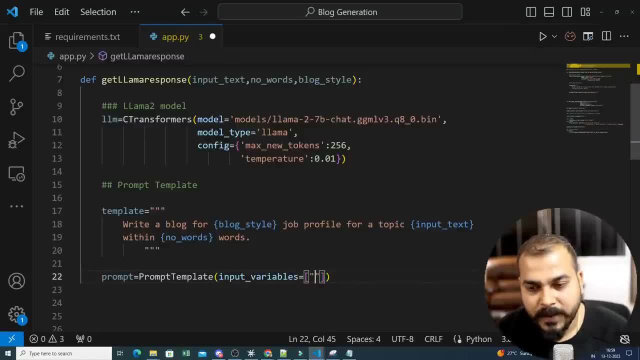 information that i want, what kind of inputs i specifically want. right, whether i want this block style. so for block style i can just write style. second one: i can probably say text. third one: i can basically say n underscore word. so this will basically be my three information. 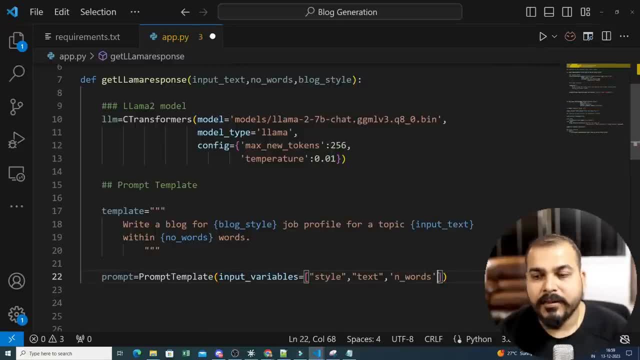 that i'm going to provide it when i'm giving in my prompt template. okay and finally, uh, this is my input variables, this next parameter that i can also go ahead with: i can provide my template itself, what template i want to give. so this will be my template over here. 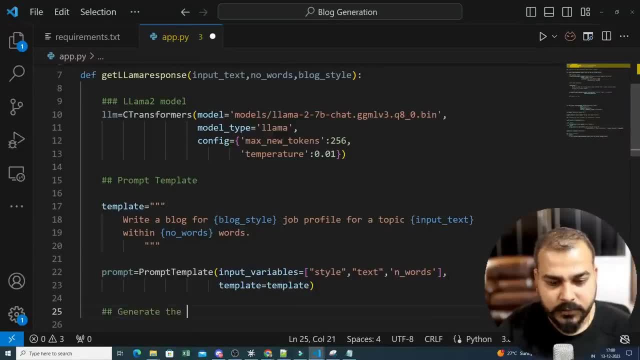 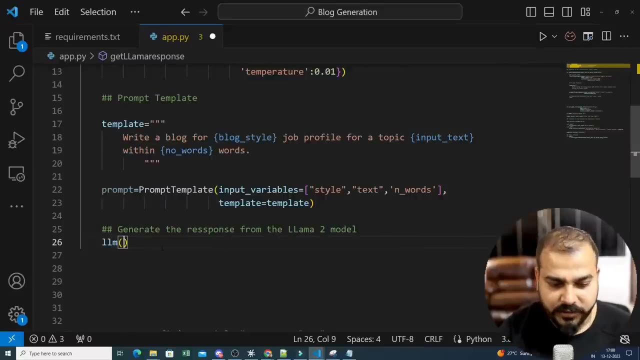 you now. finally, we will generate the response from the lama model. okay, lama 2 model, which is from ggml. okay, so here what i'm actually going to do. i'm going to basically write llm and whatever things we have learned in langchain till now: prompt, dot, prompt dot format. and here i'm going. 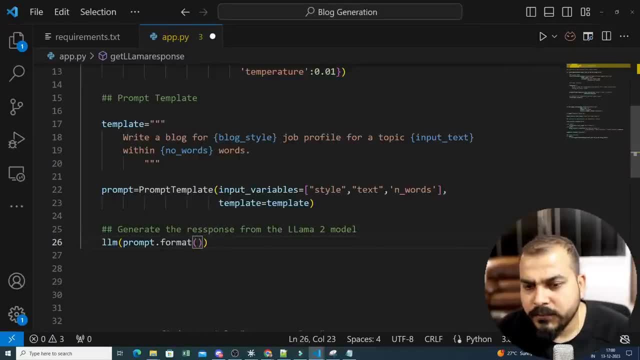 to basically use email. sorry email, no. what is the information that i really want to give over here? prompt dot format. so the first thing is with respect to style, the style will be given as block style, so i'm going to basically write blog underscore style: okay, the next information that i'm probably going to give is my input text. 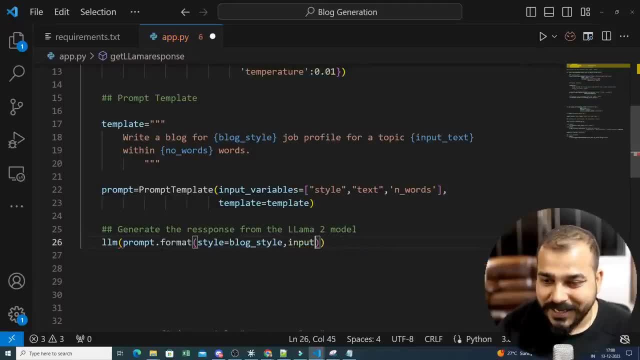 input text is equal to not input text. text is equal to input text i have to give text is equal to input underscore text and the third parameter that i am going to give is my n underscore words i'm going to give is to input Mojo use lowercase words, which will become 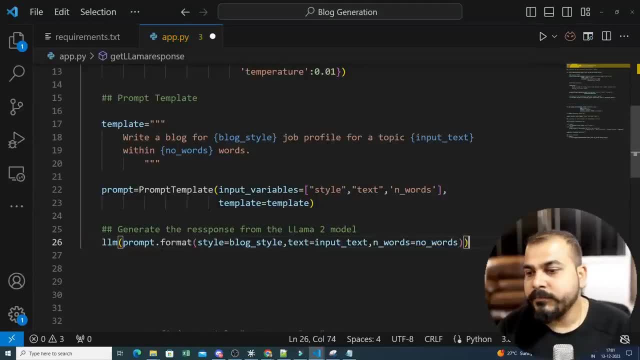 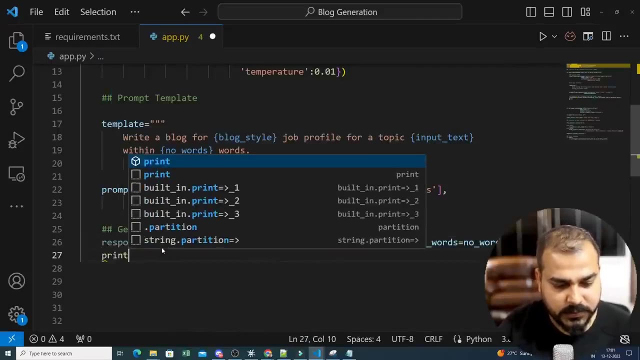 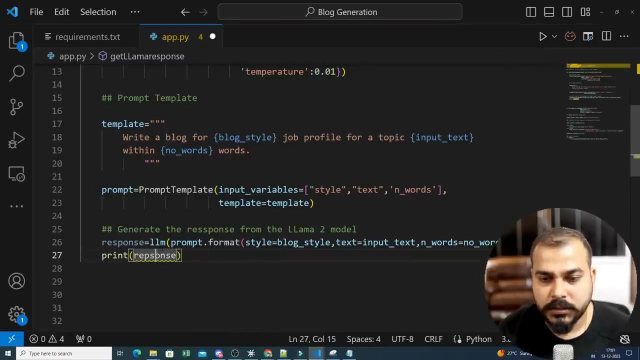 be by number of words done. so this is what I am specifically giving with respect to my prompt and what LLM will do. it will try to give you the response for this and then we will go ahead and print this response and we will return this response also. okay, response response okay and what we'll do. we will. 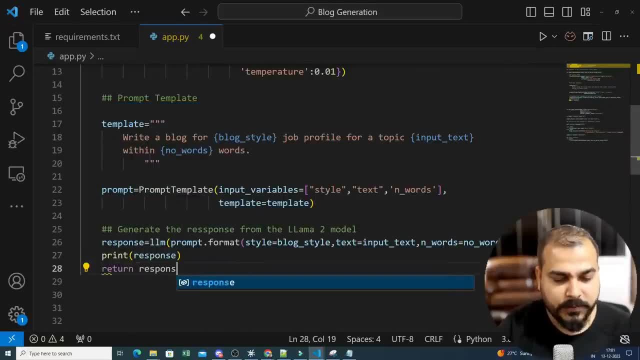 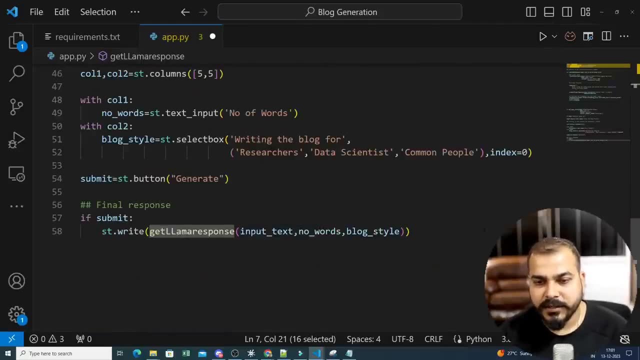 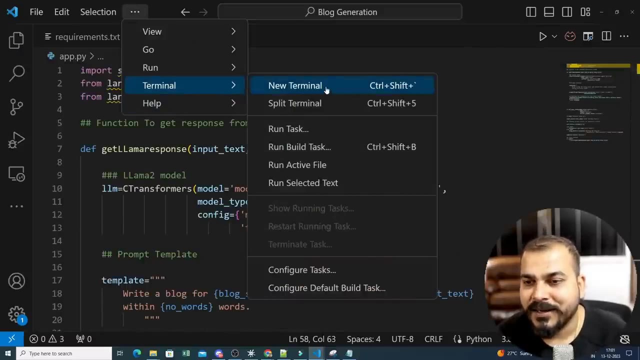 go ahead and return this response. so, step by step, everything is done. now I'm going to call this: get llama response over here. already is done. now let's see if everything runs fine or not. hope so. at least one error will at least come, let's see. so I will delete this and let's go ahead and write over here to. 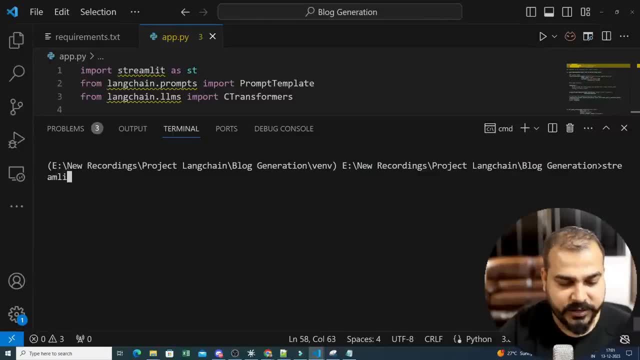 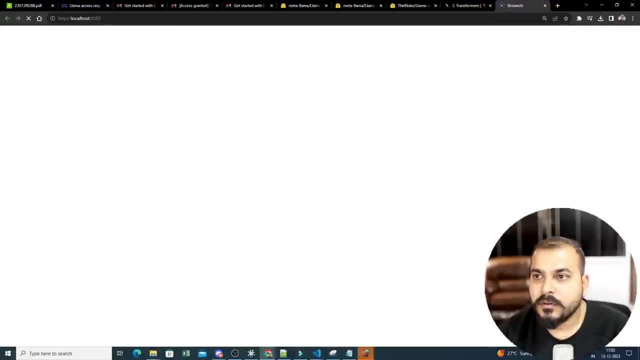 run the streamlet app. all you have to do is just write streamlet run app dot device. okay, so once I probably execute this, you'll be able to see. this is what is my model. but still, I'm getting a module. streamlet has attribute, no head, okay so 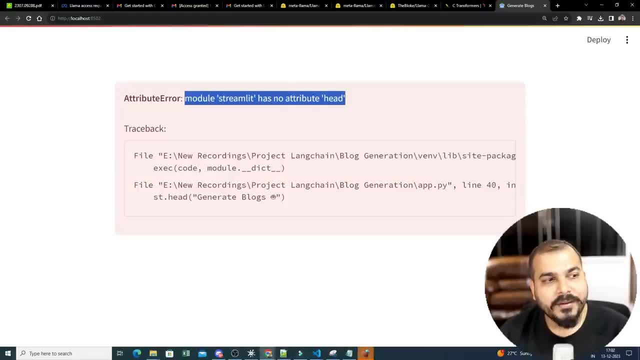 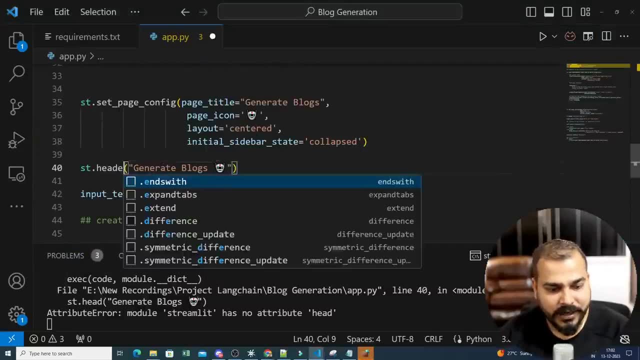 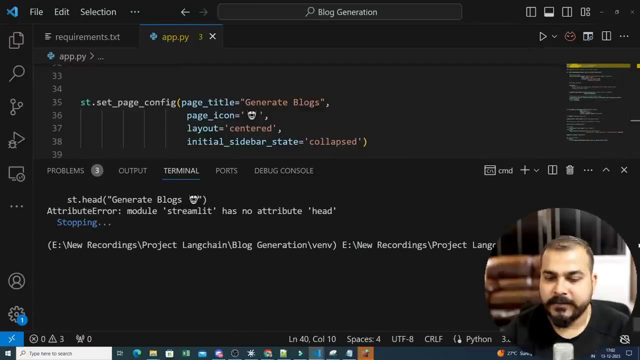 let's see where I have specifically done the mistake, because I think it should not be head, it should be header. okay, I could see the header header. okay, fine, no worries, let's run it, baby. let's run this again. streamlet run app dot py. no, I think it should run this. 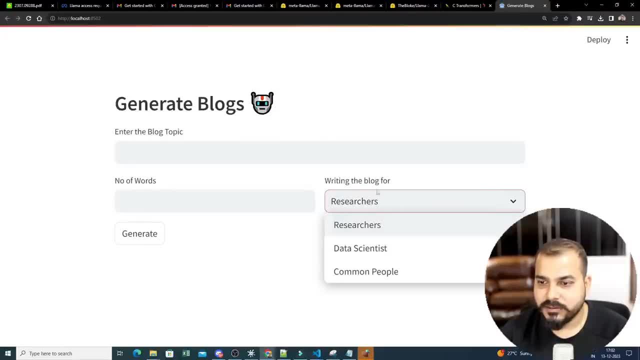 looks good. enter the blog: topping number of words: researcher, writing the researcher, blog: data, scientist, common people. so let's go ahead and write about large language model. so 300 words. so number of words: I will go ahead and write 300. I want to basically write it for common people and 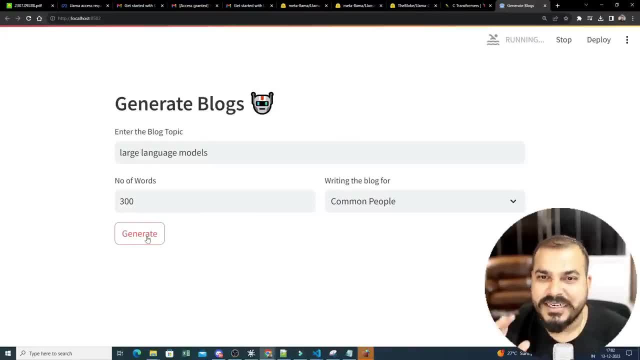 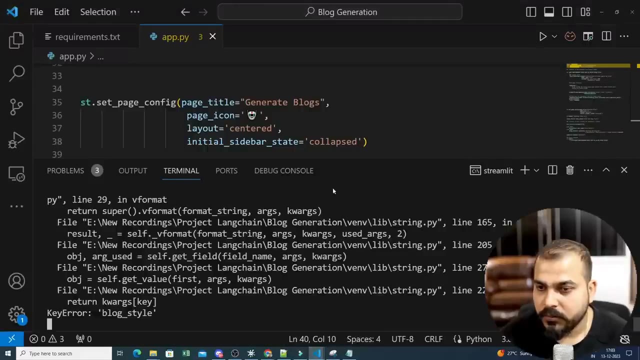 we will go ahead and generate it. now see, as soon as we click on generate, it is going to take some time. the reason it is probably going to take some time? because we are using this particular in my local cpu. but have you got an error? let's see here: rider blog, toilet Sims. so I will go to my code. 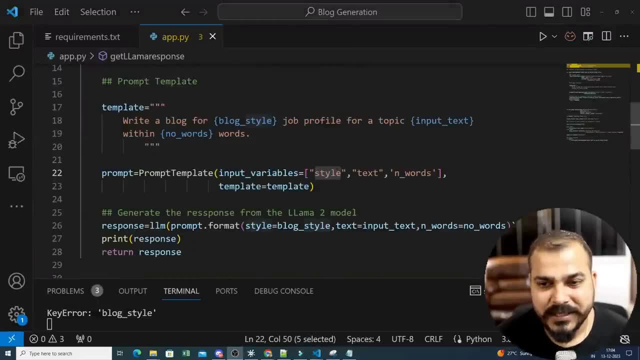 block style: blog style- blog style. so one minor mistake that are specifically done over here. so what I will do is that i'll give the same key name so that it does not give us an issue. ok, so it will be my input text: number of words. the thing is that whatever things I give in that prompt template, the input variables should be of: 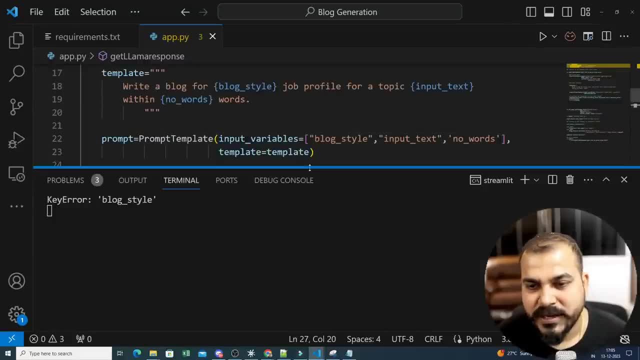 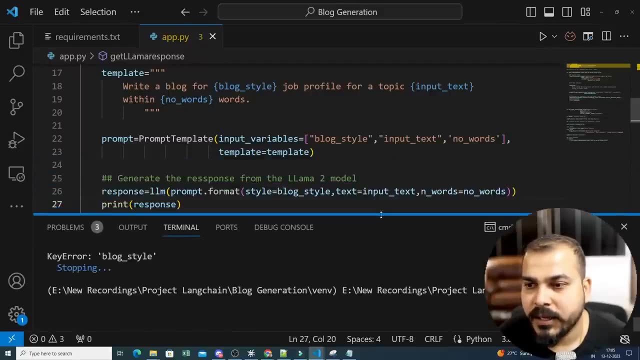 that same name. okay, so that is a mistake I had done. it's okay, no worries, so let's go ahead and execute it now. everything looks fine. have assigned the same value over there- number of words, number of words- so here also I'll go ahead and write number of words. block style input text. 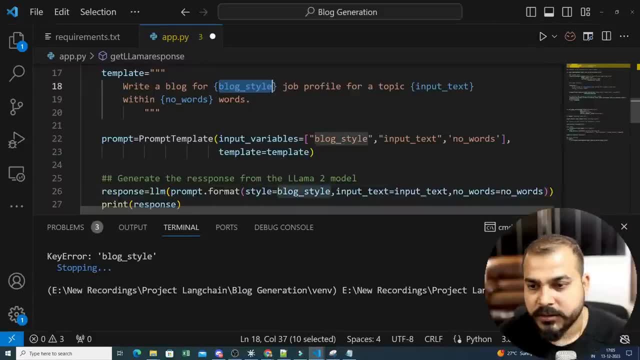 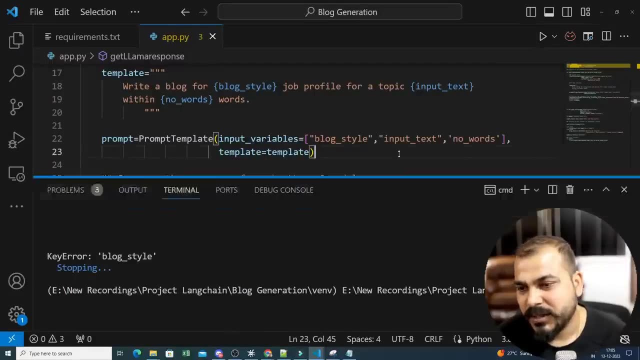 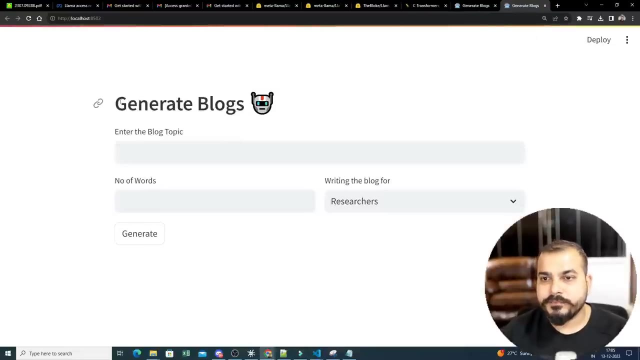 and this also should be block style the name. I'm giving same right for both prompt template and this. okay, so I think now it should work, let's see. so go ahead and write this. and now my page is opened. now I'll go ahead and write large language models and it will probably create my 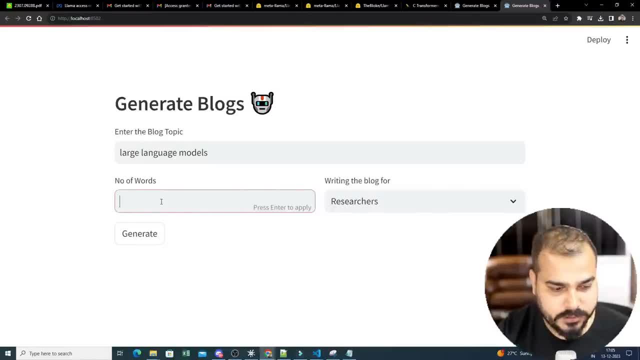 words, so this will be 300. I want to create it for you, common people, let's generate it. as I said that the output that I'm probably going to get is going to take some time because I'm running this in local CPU. let's say, if you deploy this in the 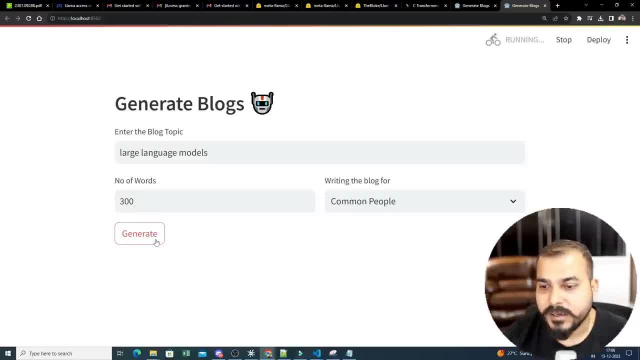 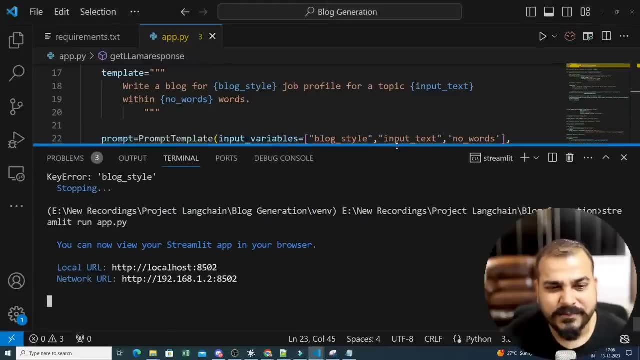 cloud with respect to if there are GPU features, then you will get the response very much quickly. so just let's wait till then. we get the output hardly, but I think it is 5 to 10 seconds max and since I've told 300 words, it is again going to take time. so let's see the output once it comes. 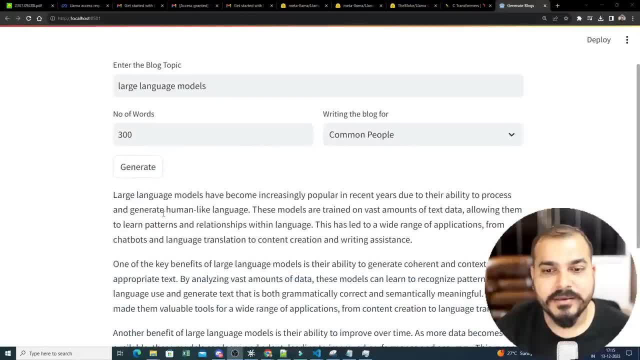 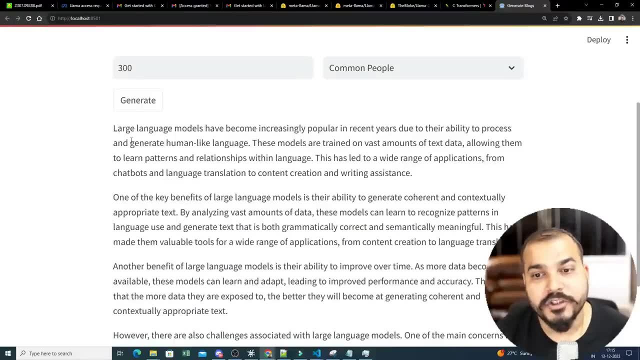 so, guys, it hardly took 15 seconds to display the results. so here you can see that large language models have become increasingly popular in recent years, due to the in, due to the ability to process and generate human-like languages. it looks like a good blog. you can also create it. any number of words block.